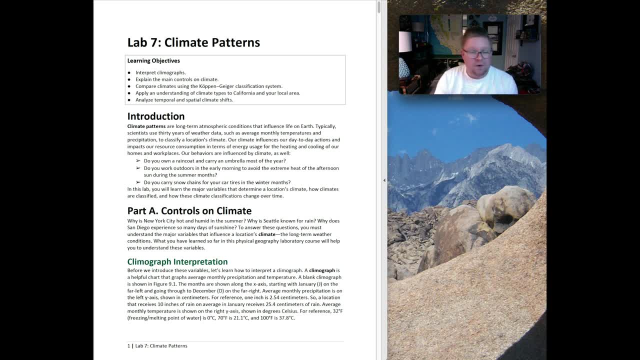 So when we say that climate is changing, we're not saying that one day is different than the next. We're saying that we have seen patterns Over decades of change, And that's a really, really important piece to understand here. So, that being said, we can see that Part A is entitled Controls on Climate. 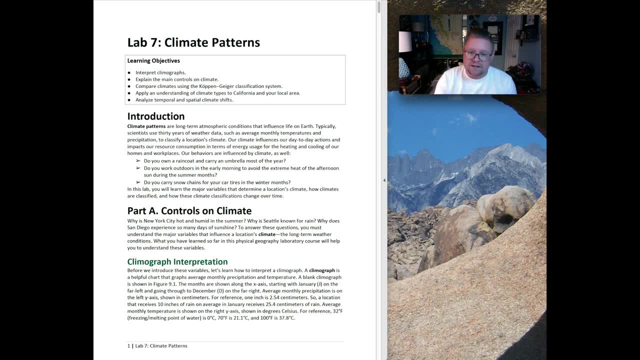 It says: Why is New York hot and humid in the summer? Why is Seattle known for its rain? Why does San Diego experience so many days of sunshine? To answer these questions, you must understand the major variables that influence a location's climate. 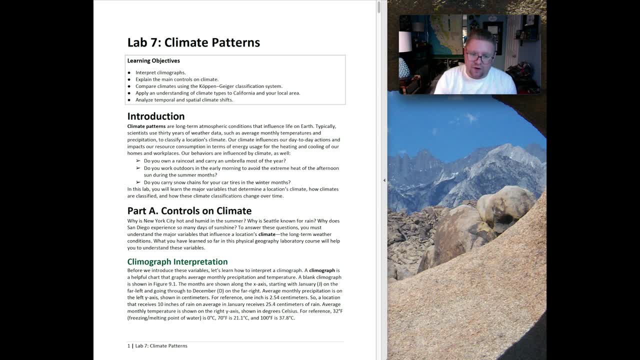 The long-term weather conditions. What you've learned so far And this physical geography laboratory course will help you understand some of these attributes. So the first thing that we can do is we can learn to interpret a climagraph. A climagraph is essentially a climate graph of long-term data. 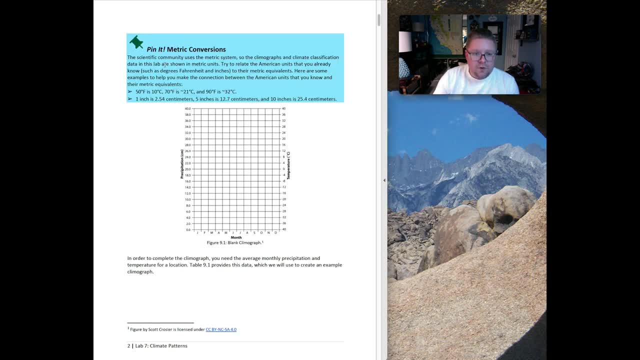 So if I move on to this next page here, we can see that it says: pin it. Here is a blank climate graph. So the scientific community uses the metric system. So climate graphs and climate classification data in this lab are going to be shown using the metric system. 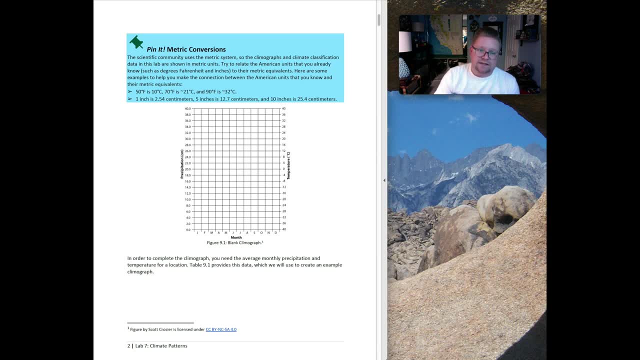 To just kind of put it in perspective: 50 degrees Fahrenheit is about 10 degrees Celsius, to just kind of put those values in order. So Fahrenheit is what we're obviously most accustomed to in the US, But in the scientific community we use Celsius, centimeters, meters and so on and so forth. 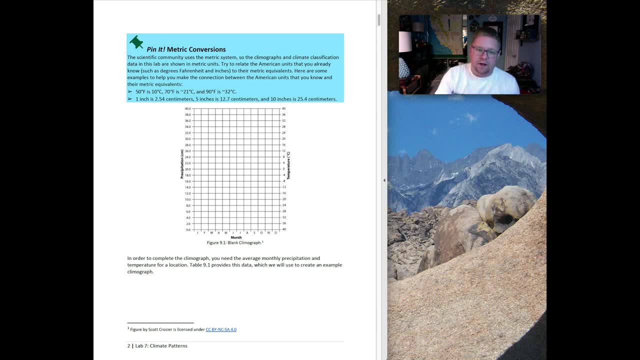 So what is important to observe about this graph- Figure 9.1, is that we can see on the bottom it has letters. Each letter or each column that might be represents a month, And then on the left-hand side, each line is represented. 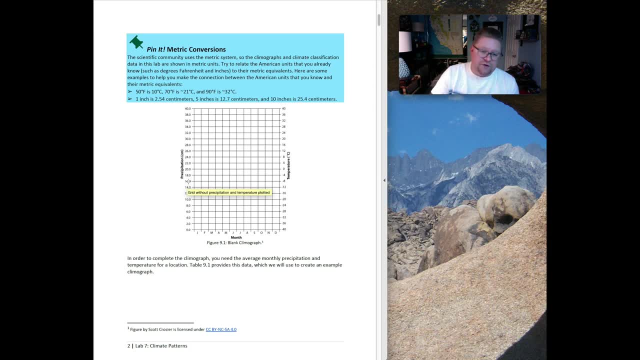 Representing a measurement of precipitation in centimeters, And then on the right would be temperature in Celsius. So what you would have is, using this graph, you could have two different elements on this graph. Mostly, it's done using a bar graph for precipitation and that's usually going to be blue. 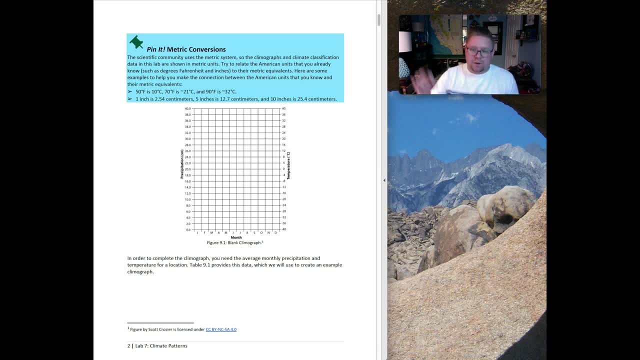 And then we usually use a red line or a different color line to represent temperature. that's been plotted And we can then observe that information. So in order to complete a climate graph, we need to have the average monthly precipitation and temperature rates for a specific location. 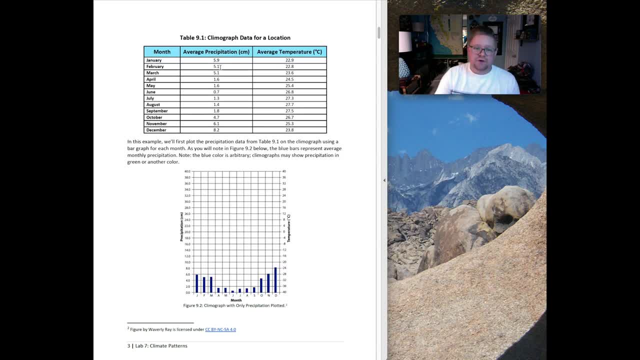 So it says here on the next page that we have that. So here we have the average precipitation in centimeters and temperature in Celsius. Now this data again is not just from last January or this January. We're talking at least 30 solid years of January. data has been put into a spreadsheet and averaged. 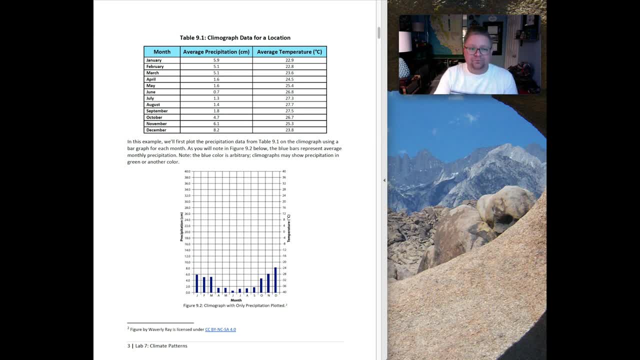 So we can look at the high and the low to get an average. So it says here in this example: we'll first plot the precipitation data from table 9.1, which is this table here- and put it on a climate graph, using a bar graph for each month to represent the precipitation. 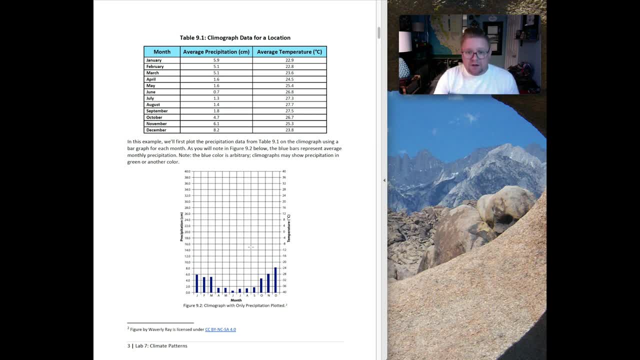 So, as you will note, in figure 9.2, below the blue bars are representing that average monthly precipitation. Note: the blue color is arbitrary. It can do just whatever you want to use, but I traditionally always use blue. So then, moving forward. 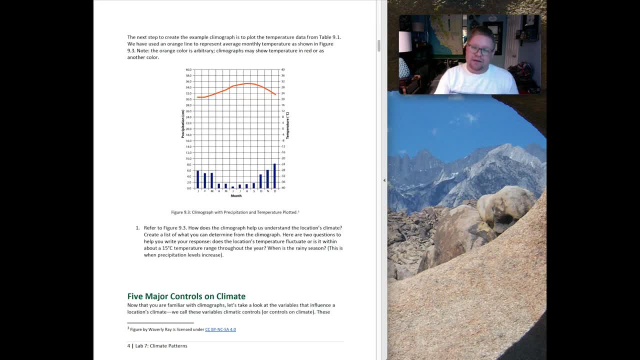 We're now able to add the next piece, which is the average temperature. So we're now able to observe a climate graph showing the average annual precipitation and average annual temperature by month. So question one says: refer to the completed climate graph 9.3.. 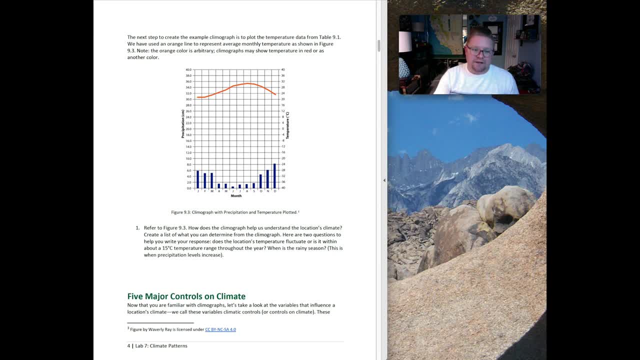 And how does this climate graph help you understand the location's climate? Create a list of what you can determine based on your observations. What can you interpret about this location based on your observations? What can you interpret about this location based on your observations? 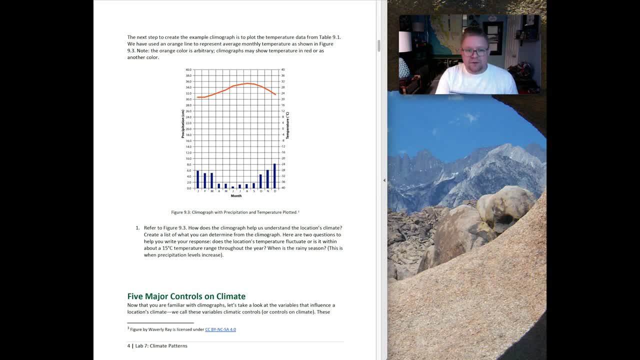 What can you interpret about this location based on your observations? How will you interpret based on these values? To kind of put things into perspective, just as a reminder, when we're talking about precipitation, about 2.54 centimeters is equivalent to 1 inch. 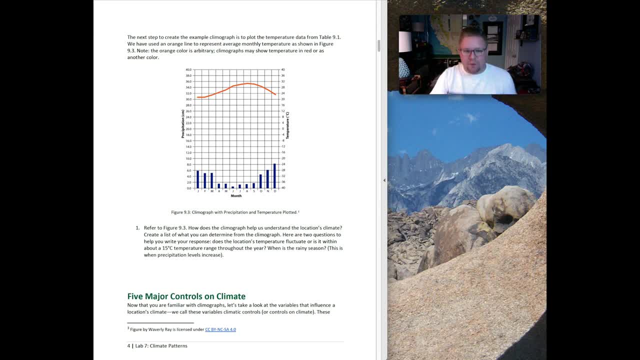 So when we're looking at just averages, if you want to put it in that perspective for your mindset, that might help you put it into a better frame of mind. Now, once you complete that, we can also look at the five major controls on climate. 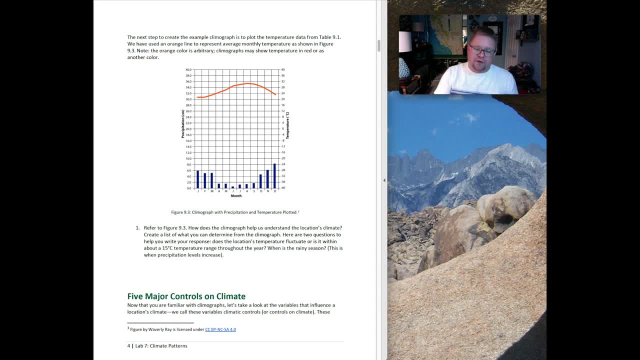 So, now that you are familiar with how to interpret climate graphs, We can now look at some of the variables that influence a location's climate. We call these climate controls. So on the next page we can see what they are. The first one is going to be latitude. 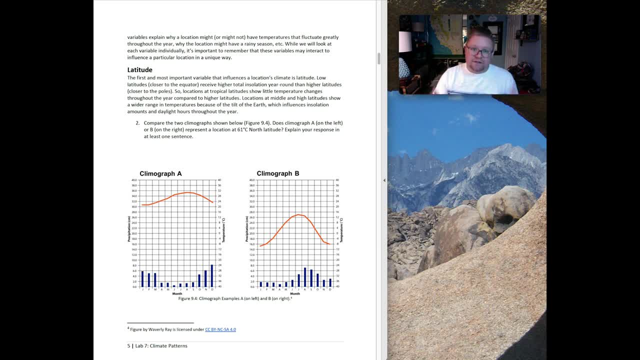 So the first and most important variable that influences a location's climate is its latitude. Low latitudes or ones that are closer along the equator receive higher total insulation, year-round or incoming solar radiation, versus higher latitude closer to the poles. 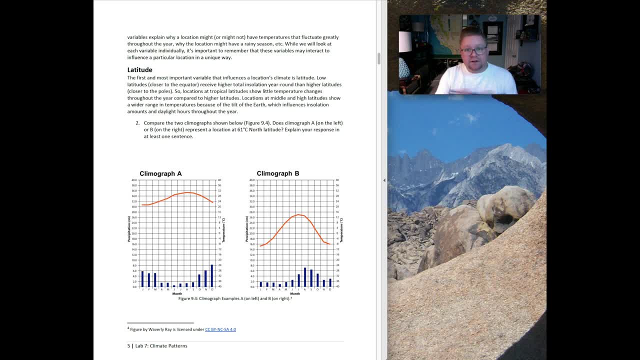 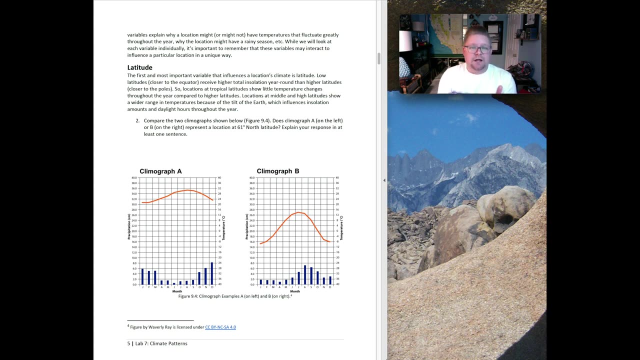 So locations at tropical latitudes show very little temperature change throughout the course of the year, While on the other hand locations of higher latitude would experience a greater fluctuation. So question two says: compare the two climate graphs below. Does climate graph A or B represent a location such as 61 degrees north latitude? 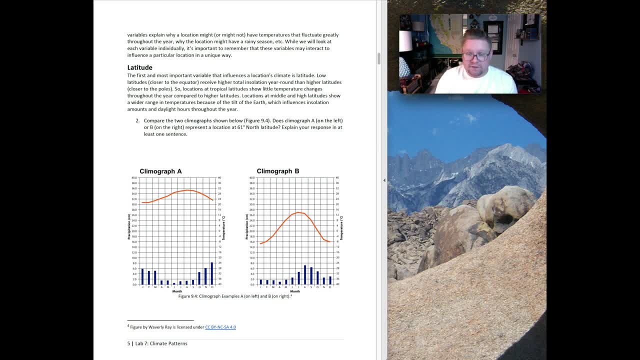 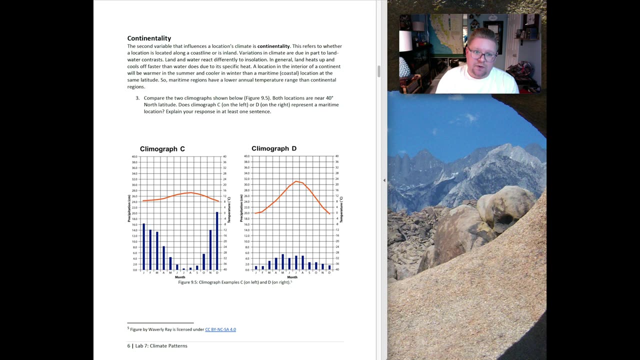 Explain your response with at least one sentence. So, based on the information provided above this lab about how latitude can contribute and affect climate, which one would you think would best represent that location? Now, continentality. So the second variable that influences a location's climate is its continentality. 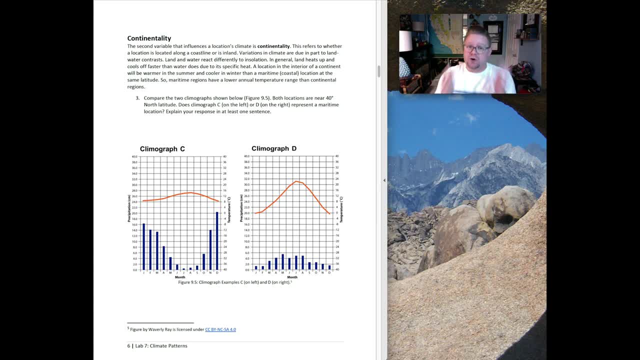 That refers to whether a location is located along a coastline or is completely inland or landlocked. Variations in climate are due in part of land-water contrasts. So as you continue working through this, question three takes you to again climate graph C. 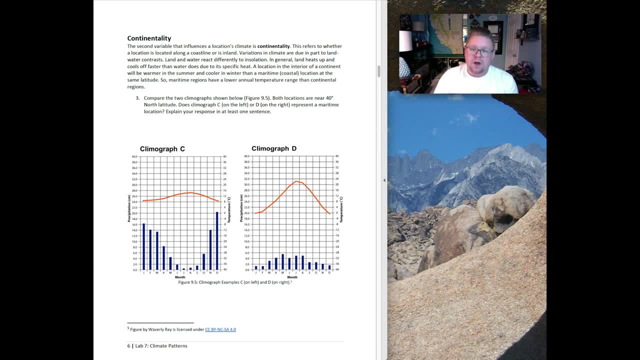 And D It says. compare the two climate graphs shown. Both locations are near 40 degrees north latitude. Which one letter, C or D, would represent a maritime location and explain why? So then, moving forward? another, you know, great effect on this would be wind patterns and air masses. 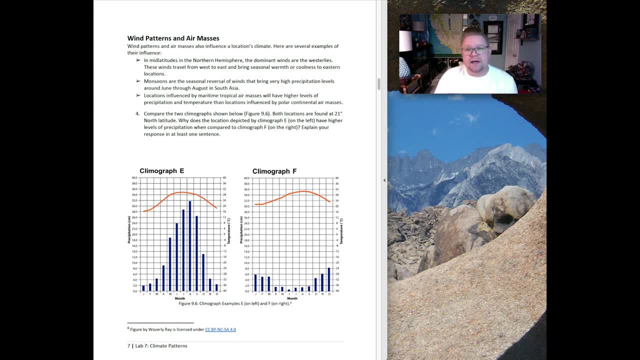 So wind patterns and air masses also influence a location's climate. Here are several examples of their influence, such as: in mid-latitudes in the northern hemisphere, the dominant winds are the westerlies. These winds travel from west to east and bring seasonal warmth or coolness to eastern locations. 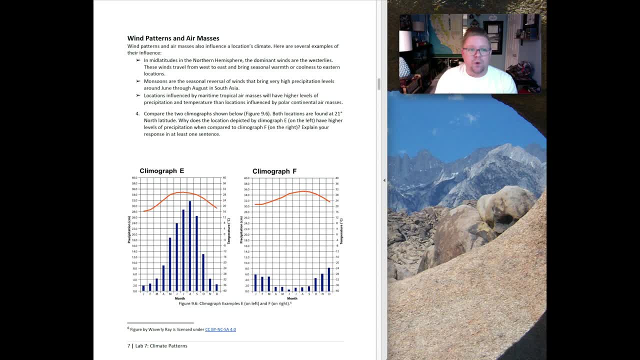 And you'll see that there's some additional references there. Moving forward, question four: Comparing climate graphs E and F. They are both located and found at 21 degrees north latitude. Why does one location depict by climate graph E have higher levels of precipitation when compared? 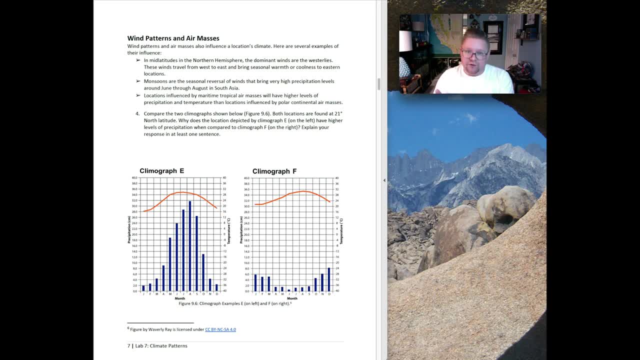 to climate graphs E and F. So again, using information that you have observed and interpreted so far in this lab, make those correlations. Why is climate graph E have exceedingly amount of precipitation versus climate graph F, although they're at the same latitude? 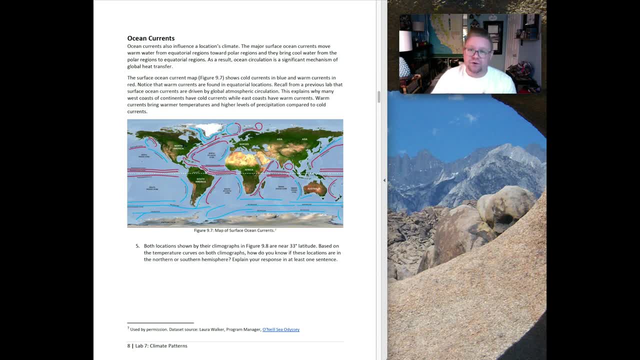 So, moving forward, we can see that ocean currents are also a contributing piece to this. Ocean currents influence a location's climate. The major surface ocean currents move warm water from equatorial regions towards the ocean And they bring cold water from the polar regions back to the equatorial regions. 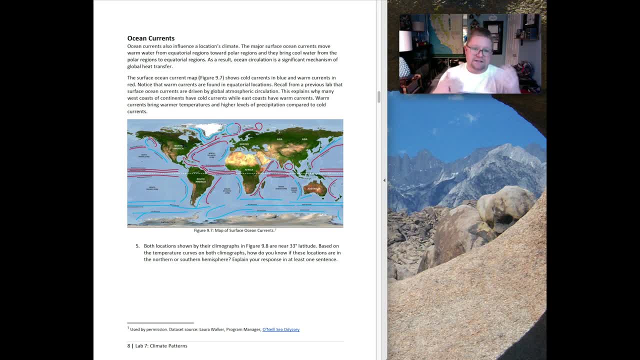 So, as a result of this circulation, it provides a significant mechanism of global heat transfer. So here we have a beautiful diagram, figure 9.7, the map of the surface ocean currents. So we can see: if you just very simplistically look at this diagram, you can see the blue and red. 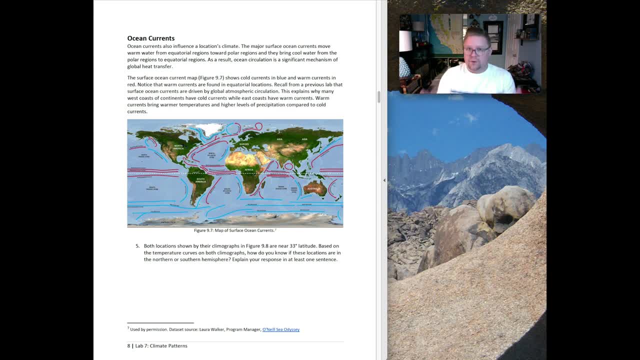 Blue is colder water, red is warmer water, Warmer equatorial blue versus polar. Look at the mixing and how that occurs. That mixing is really working towards equilibrium. It's so important that this occurs. So question 5 says: okay, let's look at a climate graph. 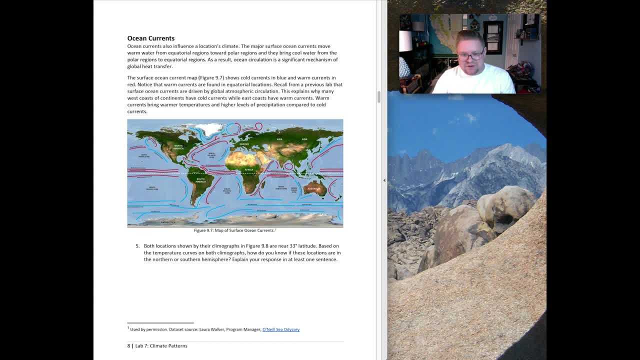 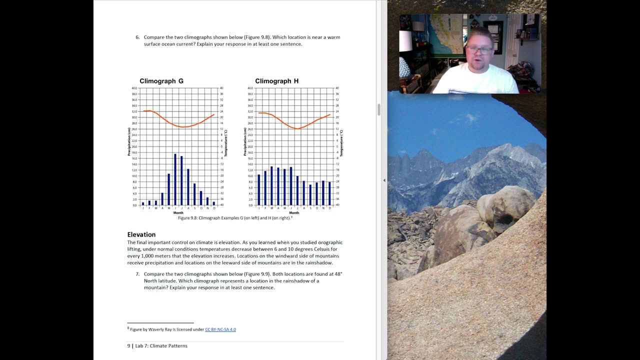 Both locations are at 33 degrees latitude. Based on the temperature curves of both the graphs, how do you know if these locations are either in the northern or the southern hemisphere? So, using this information and looking at these climate graphs, which one do you think would be in the northern versus the southern hemisphere? 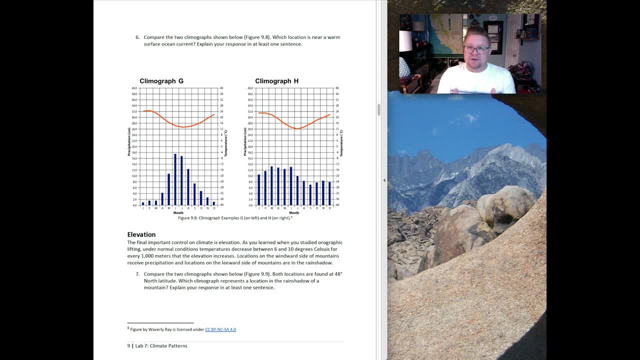 Something that's very helpful when understanding that is, think about this: A majority, nearly 70% of all the land mass of our planet is found within one particular hemisphere. That might be helpful for you when trying to solve that question. And then question 6 says: comparing the two graphs below: 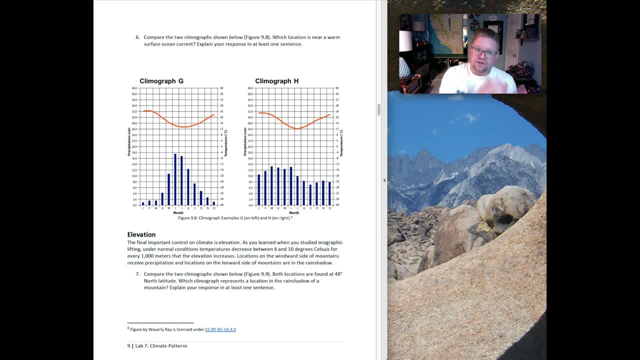 which location has a warm surface current and explain why Another contributing factor to how climate really is distributed across our planet will be the elevation right, That altitude. So it says the final important control on climate is its elevation, As you learned when you studied orographic lifting. 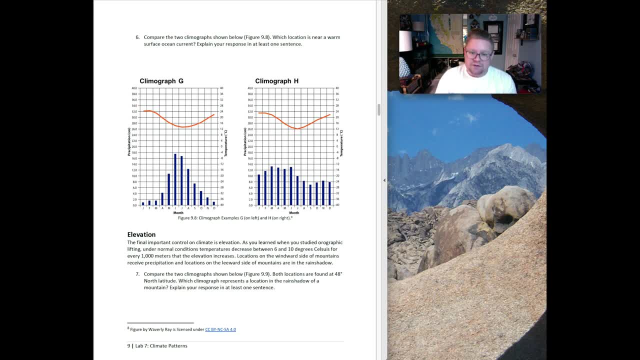 under normal conditions, temperatures decrease with altitude. So, that being said, question 7 says: comparing the next two climate graphs shown figure 9.9,. both are found at 48 degrees north latitude. but which location would represent a location in the rain shadow of a mountain? 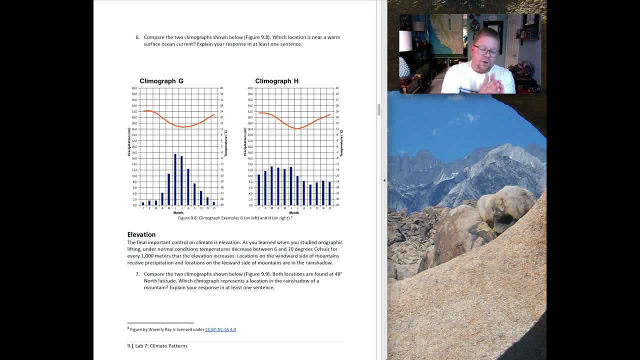 Remember When you learned about orographic lift. one side will have a majority of that precipitation because as the cloud gets lifted up, it gets cooler, there's less pressure, the condensation occurs and precipitation can occur, and then the cloud goes over the mountain, sinks back down. 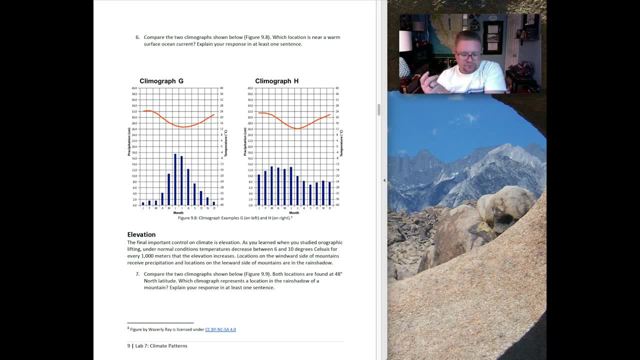 and it gets warmer due to atmospheric pressure. It's heat by compression. So, that being said, one side is usually wetter and the other side is drier. So, looking at these next climate graphs, are we able to make some form of observation? 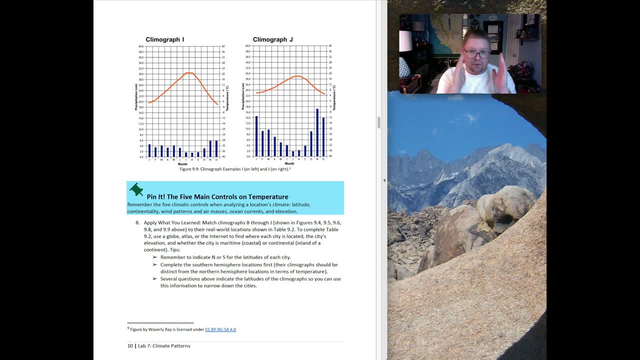 which side would be of which. So now we plug into a pennant the five main controls of temperature. Remember, the five main controls of temperature, when analyzing a location's climate, will be its latitude, continentality, wind pattern, air mass, ocean currents and its elevation. 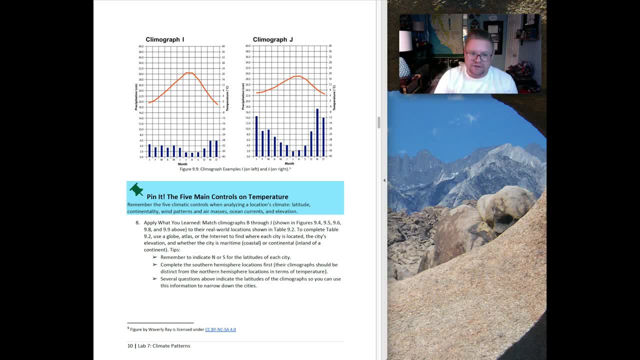 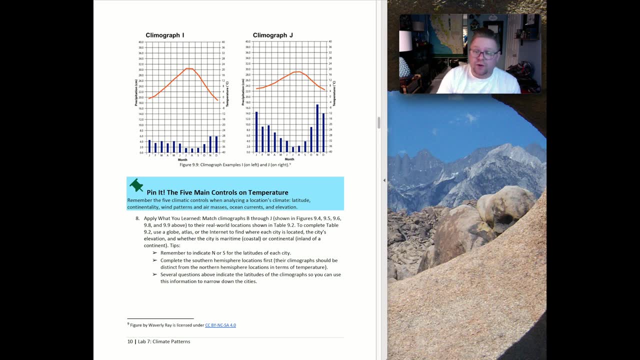 So question 8 kind of brings everything together. It says: now apply what you've learned. Match climate graphs B through J to their real world locations shown on tables 9.2.. Now to complete the table, use a globe or atlas or the internet. 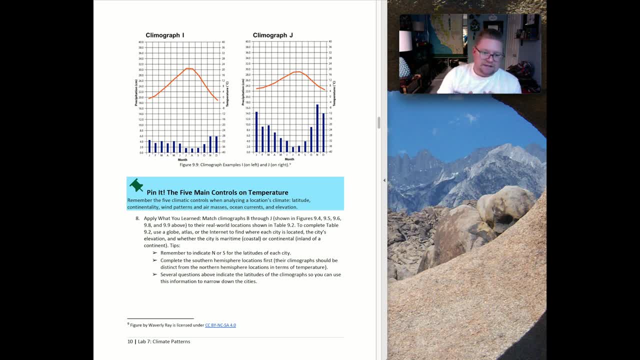 to find where each city is located Is the city's. you know what its elevation is, whether the city is maritime, continental, so on and so forth. It does provide some additional tips. So, again, that's going to be climate graphs B. 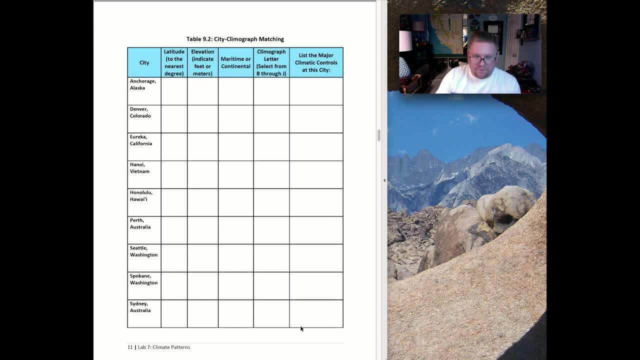 as in boy through J, And then you have them here. So these are our random locations. You're going to match those up and then, once you've matched them up, you're going to be able to include the latitude to the nearest degree. 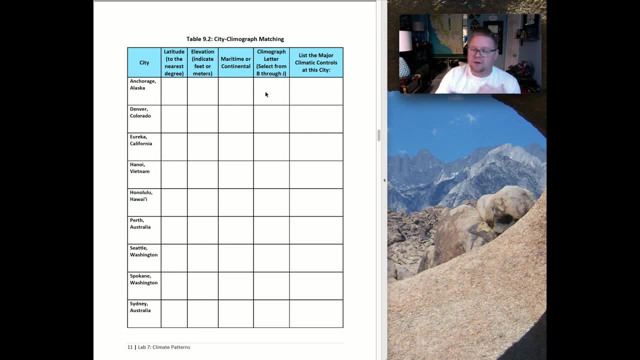 the location for that location, Is it maritime or continental? The climate graph letters, section from B through J, and the list of the major climate controls in that city Based on those five climate controls. write down the major climate controls of that city. Now the climate graph letter. 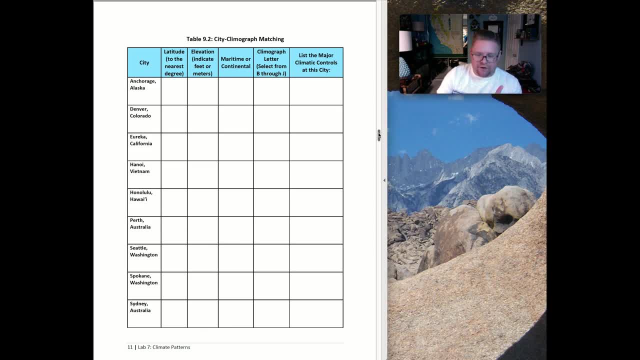 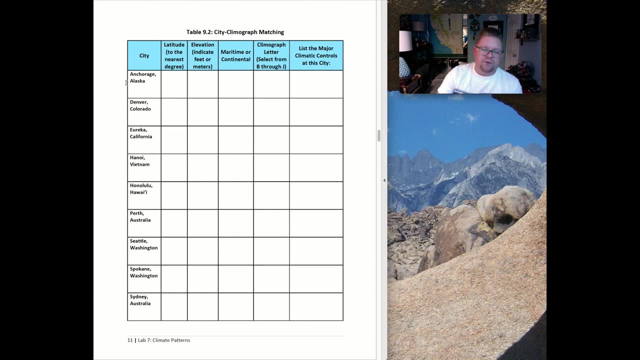 it says selected from B to J is a little bit different. When you're looking at these climate graphs you're going to see the letters, So you pick the letter that goes there. So that way we know. okay, so if we decide that Anchorage, Alaska, is letter B, 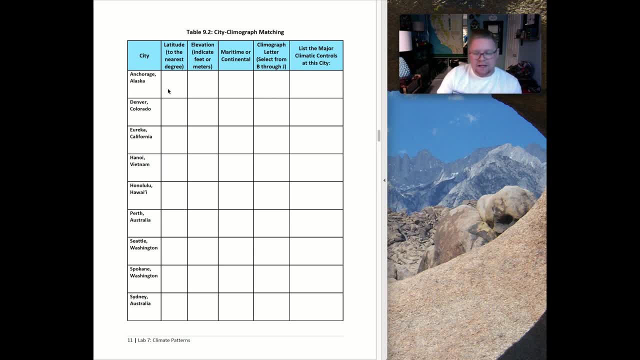 you would write letter B there And the key is I would do it in pencil first, So that way, in case you make mistakes, you can move it around. But I think what would be of most help first is to really just sit there and find out. 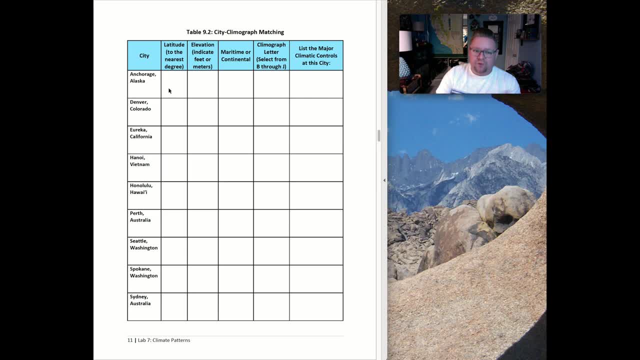 what is the general latitude- north or south- for each of these locations, And when you're doing that, try to find out what its average elevation or altitude is, so you kind of have an idea there. Then you're going to be able to match them. 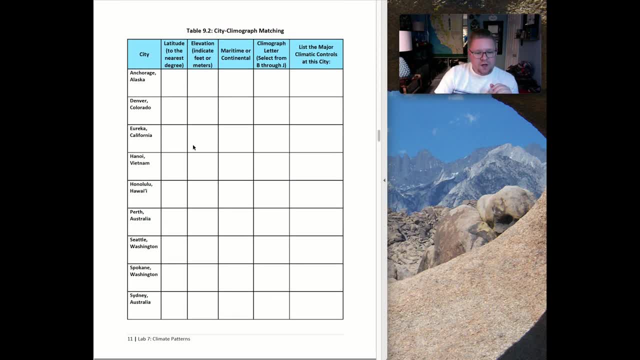 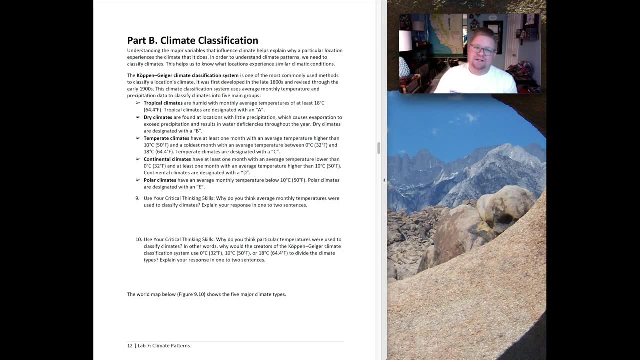 and I think it's going to make it so much easier for yourself. But anyway, that being said, that wraps up part A. So part B is called climate classification. Now, being able to do this is really helpful. I think it really allows you to generalize. 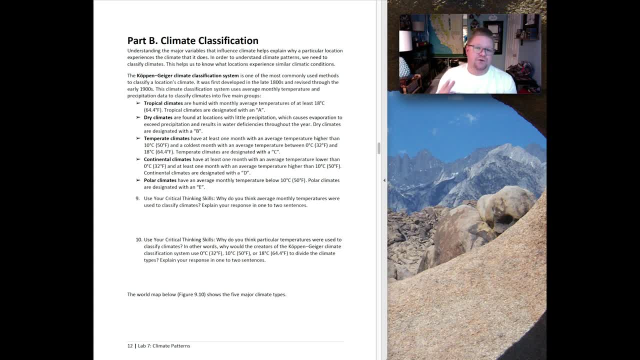 and to understand regions. But many geographers or scientists will argue that this is not always the best way to do it because of certain examples. Small places, small states, not a problem, It's usually the same weather and climate on both sides of those areas. 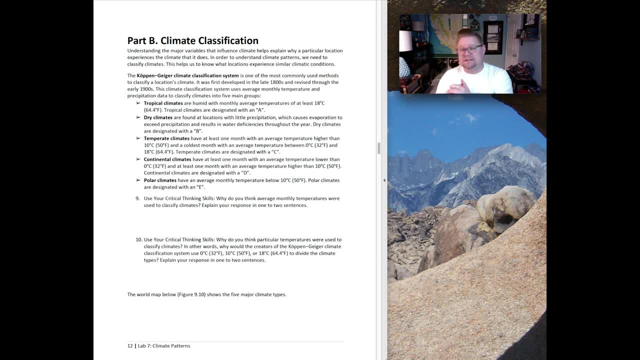 and there's not a lot of variation. But places like California, as an example, the weather can be very, very different. The general climate is very, very different compared to San Diego versus San Francisco, So it becomes challenging if you want to be able to give California. 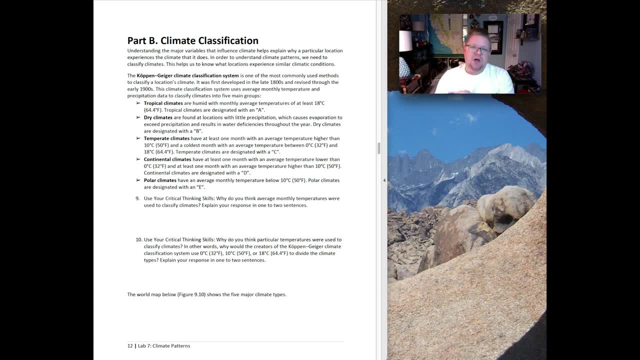 just one climate classification. It's impossible. We have to do it in regions. But other states can be done. An entire state can be classified, But what this does is it takes all that data and creates a generalization. So I always give this example in my class. 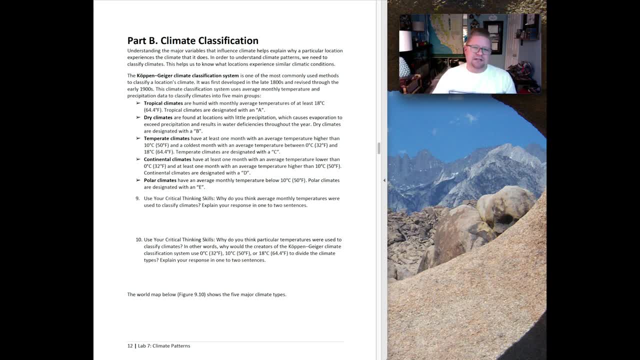 Imagine that I'm going to pay an all-expense-paid trip to Las Vegas in July, but you have to pack now. Whatever month it is, it doesn't matter what it is, you have to pack this early on. Could you do it? 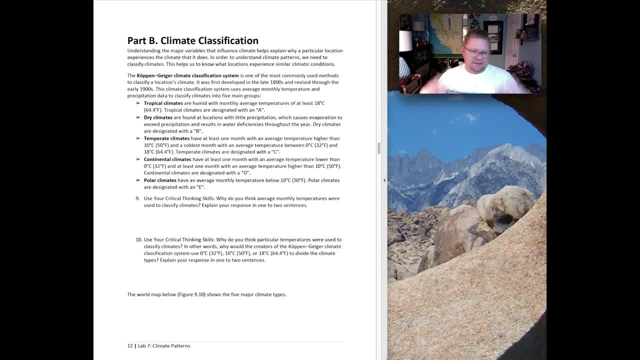 And the answer is, of course you could. It's going to be Las Vegas in July. It's going to be hot. I mean, could it rain? It's possible They do get freak summer storms out in Las Vegas, but we know it's generally going to be bathing suit weather. 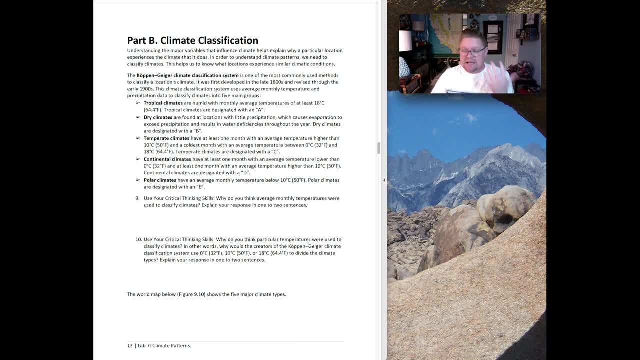 because we're able to take long-term understanding and data of that region and to create that classification. So that's really how this works, So the way that this works, which is, again, one of the most popular methods that is done, and we've been using it forever. 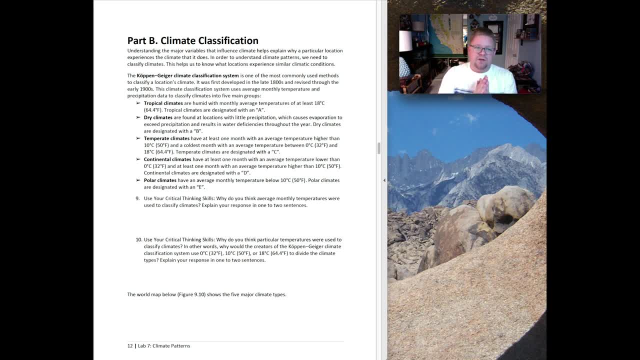 is that we first start off into like tiers. We start with the basic climate group and then we can break it up into temperature and stuff like that. So it says here to understand, to begin, that these are our general climate areas. We've got tropical, dry, temperate, continental and polar. 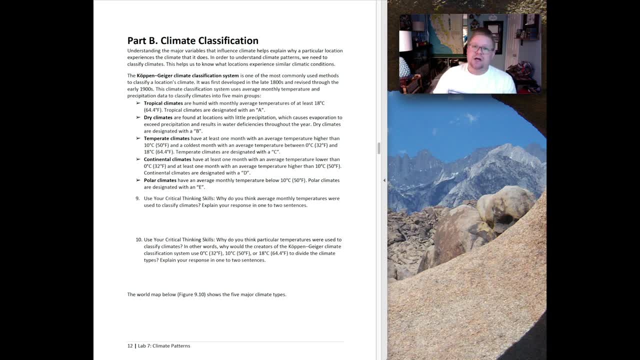 Now each one of those regions has been denoted a letter. So tropical climates will begin with a letter A, a capital A. Temperate climates will be given a capital C, and so on and so forth. Now, using your critical thinking skills. 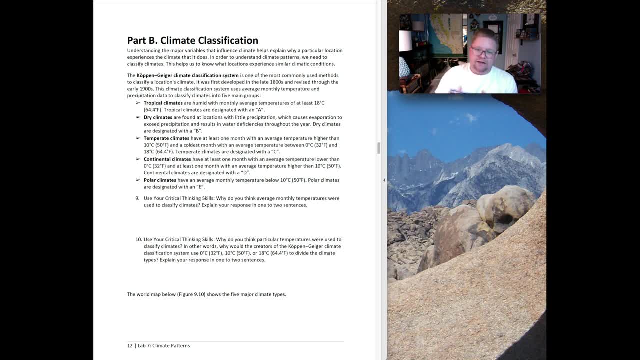 why do you think average monthly temperatures were used to classify climates? So, based on what you've observed about these different region areas and types of climates, why do you think that the average monthly temperatures are so important when coming to this idea? Question 10 says: 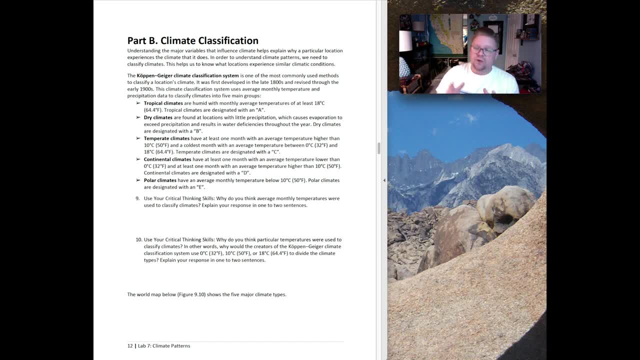 using again your critical thinking skills. why do you think particular temperatures were used to classify these climates? In other words, why would the creators of the Copenhagen Climate Classification System say that you know? use 0 degrees Celsius, 10 degrees Celsius, 18 degrees Celsius. 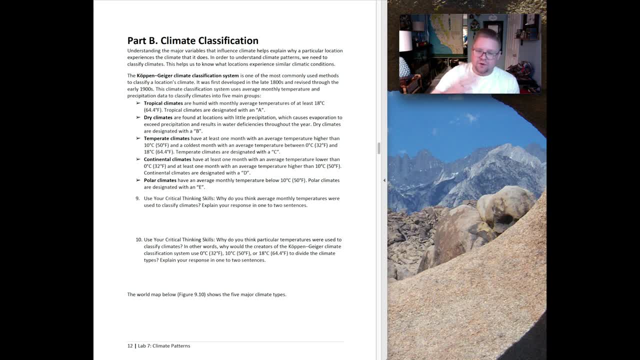 to divide the climate types. So what are those breaking points? What does 32 degrees Fahrenheit really mean? What does 50 degrees Fahrenheit mean, And so on and so forth? There is a reason why those numbers were chosen, and kind of think about it. 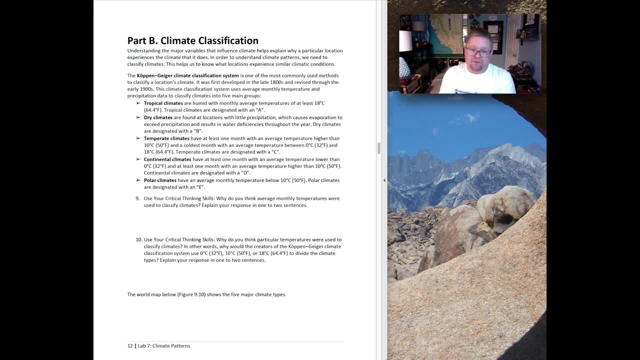 I mean, I don't know, when I think about stuff like this, I put it in perspective. You know what? you have probably experienced 32 degrees Fahrenheit. You've probably experienced 50 degrees or 64.. What does that mean for you? 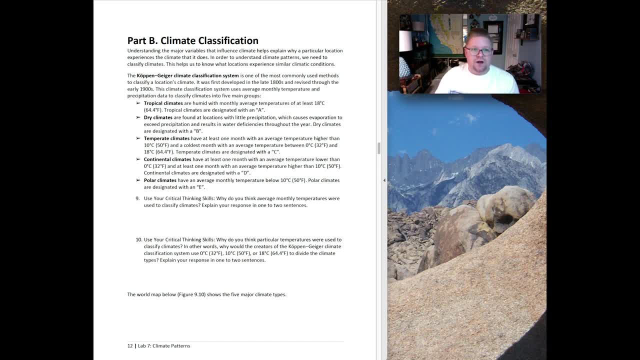 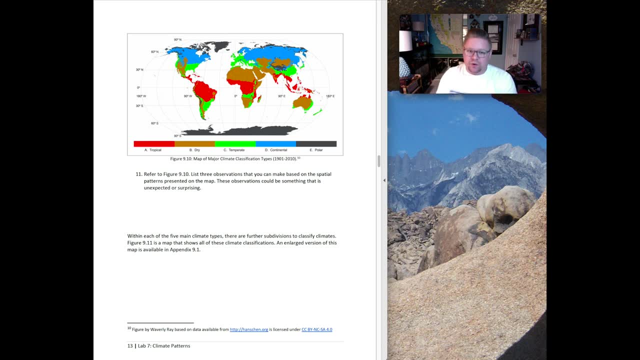 Now moving forward. the map below figure 9.10 is a very generalized climate map showing the average climates between 1901 and 2010.. So we can see this is broken up as just tropical, dry, temperate, continental and polar. 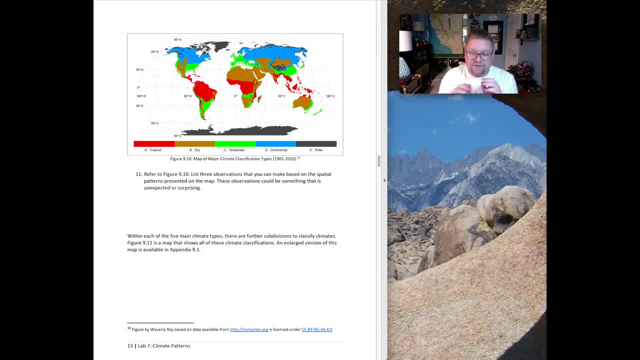 Very simplistic. We'll dive a little more into. you know, essentially you segregate each one, You subdivide tropical areas a little bit smaller, but for now big picture. So figure: 9.10,. this is question 11.. 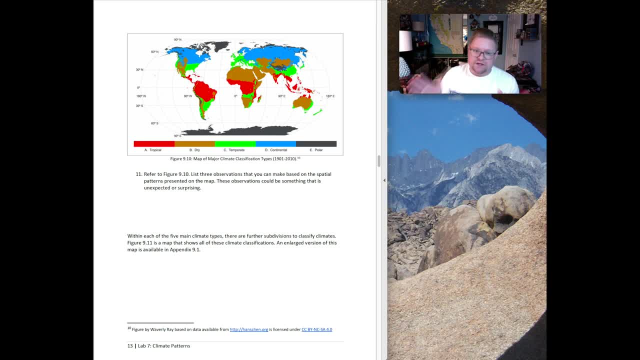 List three primary observations that you make based on the spatial patterns presented in this map. These observations can be something like this, Something that is either you know, unexpected, surprised, or maybe even you expected something like that. So you know, is there correlations? 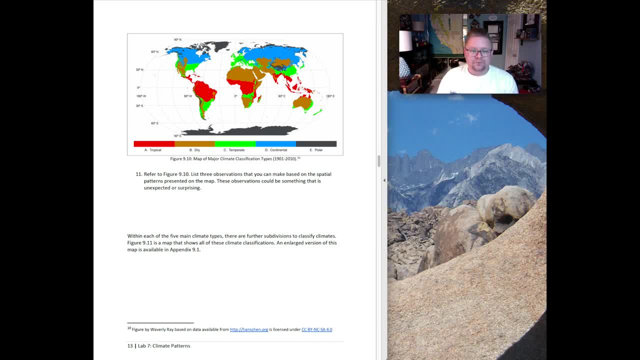 Are there any patterns that you observe in this map? So then it says: within each of the five main climate types there are further subdivision climates. Figure 9.11 is a map that shows all of them put together. It's that putting it together piece. 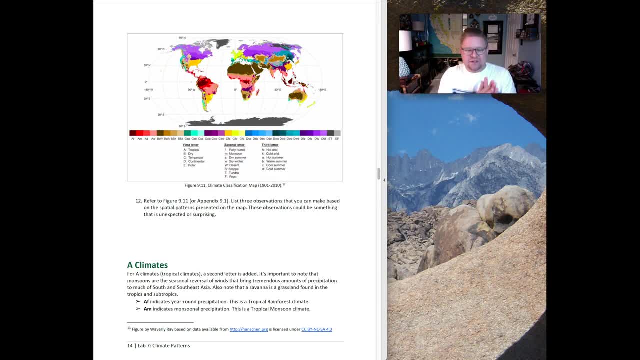 See, it got a lot more complicated, So we can see that there's different options. It's like a color spectrum, So we have our A, B, C, D and F, you know, and E- sorry, E again. 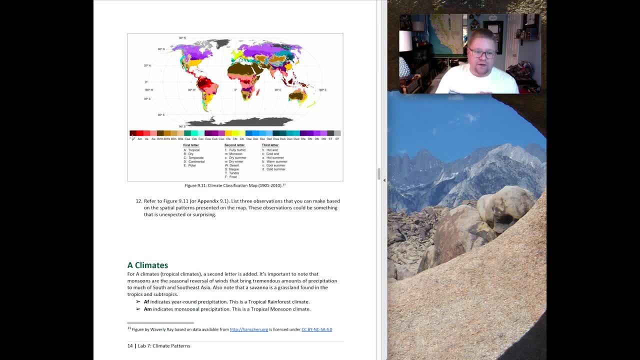 But now we have subdivisions. You know, we have one that's a capital, A lowercase f. Well, what does that mean? That means it's a tropical area that is fully humid. We have an area that's, as an example, CFA. 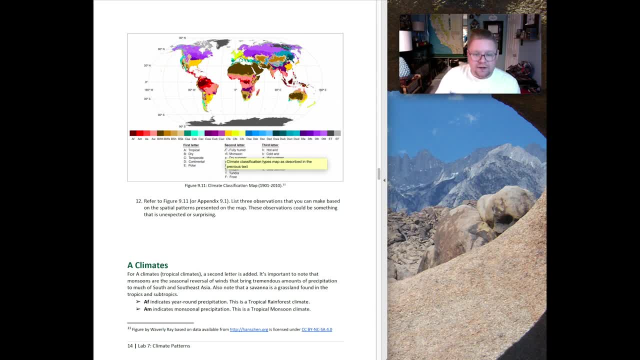 That means it's a temperate, fully humid, and it's also going to have a hot summer. So there's a pattern in which we follow. So question 12 says: refer to figure 9.11.. List three observations that you now make. 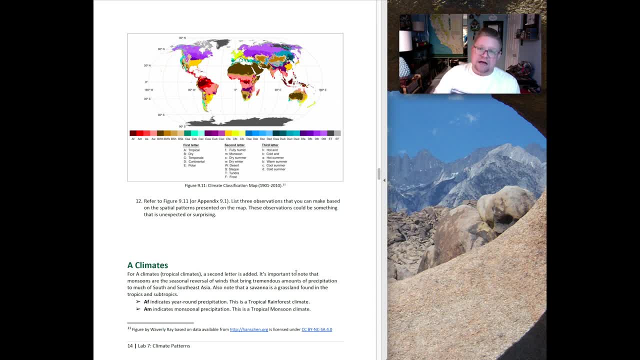 based on the spatial patterns presented in this map. Now this map is more fine-tuned. You know these observations can be something that is unexpected or surprising, So let's break each climate group, Let's talk about that and all the options within. 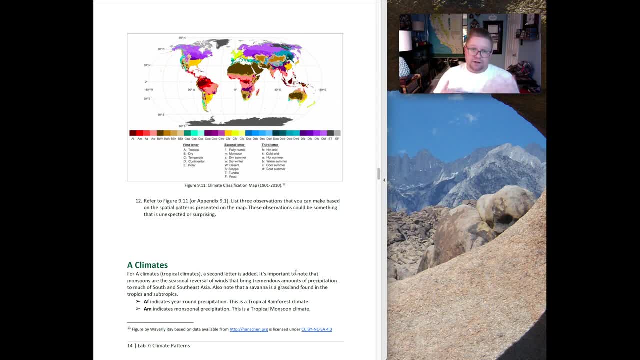 So, as we can see, for climate A, which are considered tropical climates, a second letter is added. Why? Well, it's important to know that monsoons are the seasonal reversal of winds that bring tremendous amounts of precipitation to much of the South and Southeast Asia. 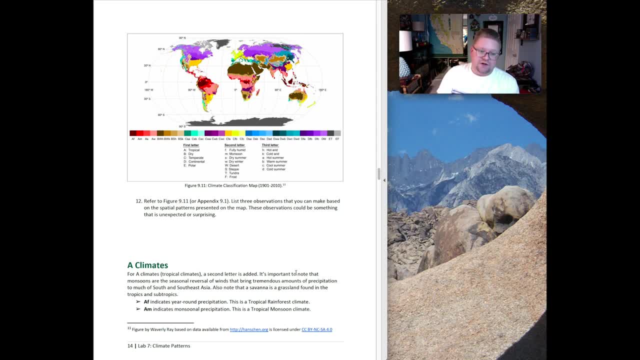 Also note that the savanna is a grassland found in tropics and subtropic areas, So we can see that if it's an AF, it indicates that it's year-round precipitation. This is a tropical rainforest, Or an AM indicates monsoonal precipitation. 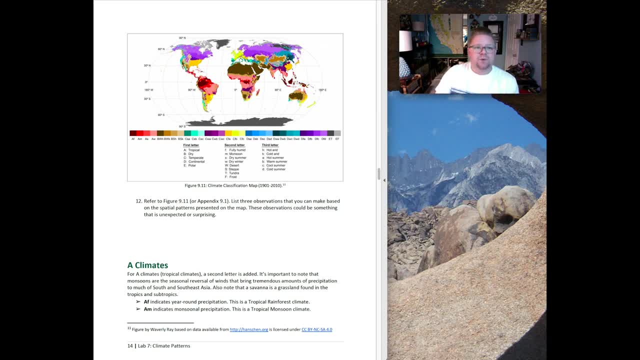 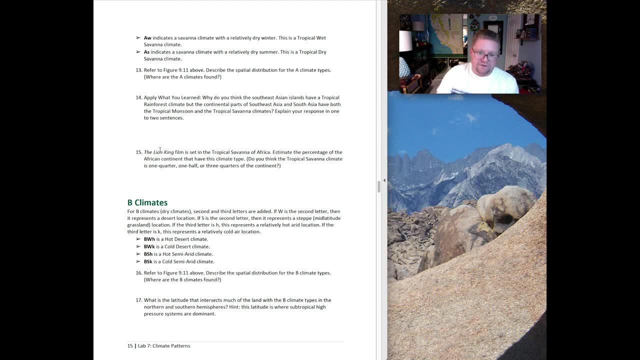 meaning that it's seasonal, So you're able to work through these different options and see what it says. Here's an option for AW and AS. So question 13,, 14, and 15 is having you look at. you know. 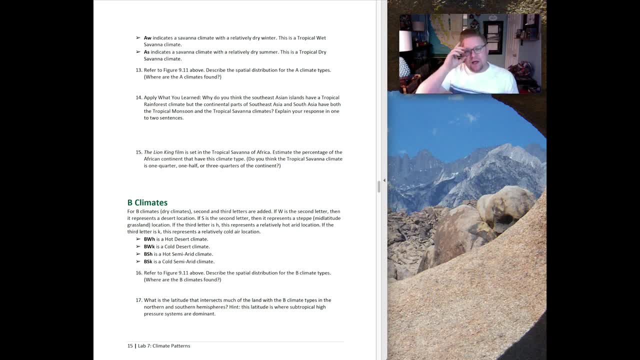 not just the figure above that big map that puts it all together, but also the very fine-tuned definition of each one of these, and answer questions. like you know, describe the spatial distribution using what you've learned. Why do you think Southeast Asian islands have tropical rainforest climates? 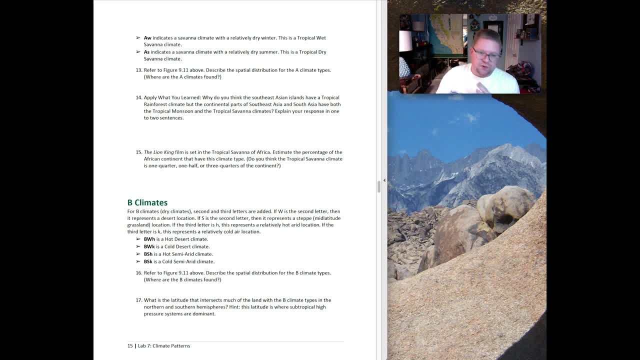 but the continental parts may either be monsoonal or savanna. And then there's a great question that kind of brings it back and talks about the Lion King and thinking about you know the climate and Lion King and where it was set and you know how does that work. 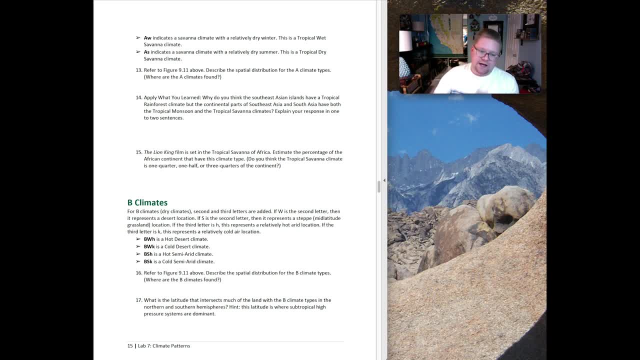 Moving forward, we can look at B-type climates. We've got again a handful BWH, you know BWK, so on and so forth. So what it says here is for dry climates. second and third letters are added. 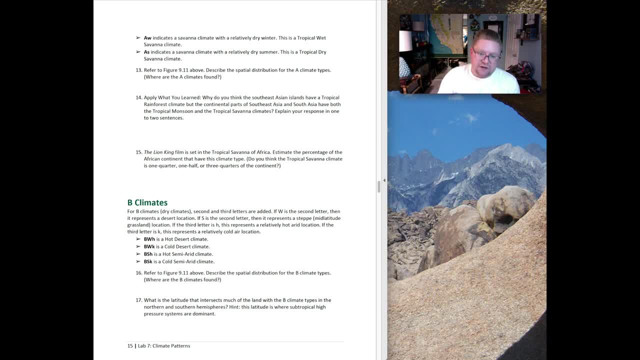 If a W is a second letter, then that represents a desert location. If an S is a second letter, then that represents a mid-latitude grassland. So again we have these codes that we kind of work in Questions 16,, 17, and 18, sorry, 16 and 17 are the same thing. 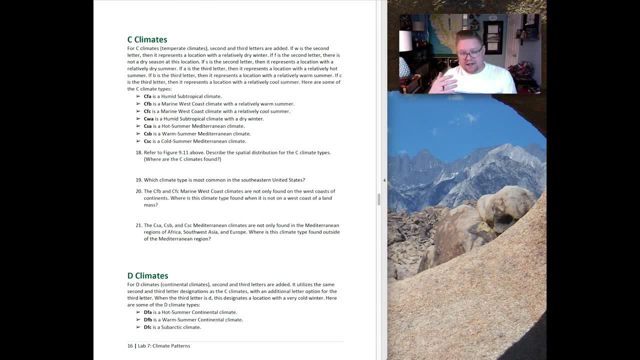 asking you to reflect on those definitions, looking again at that map. Same thing for climate C. I live in Santa Clarita, so this is our dominant climate. Here is a C. We're actually a CSA. We are considered a hot summer Mediterranean climate. 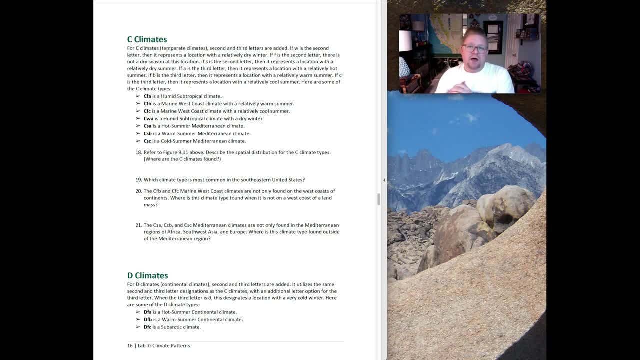 which makes sense, because here in Santa Clarita we get like two days a year that are really cold in January. Otherwise you can pretty much grow vegetables and produce all year round. here in Santa Clarita We do have not crazy humidity, It's more Mediterranean. 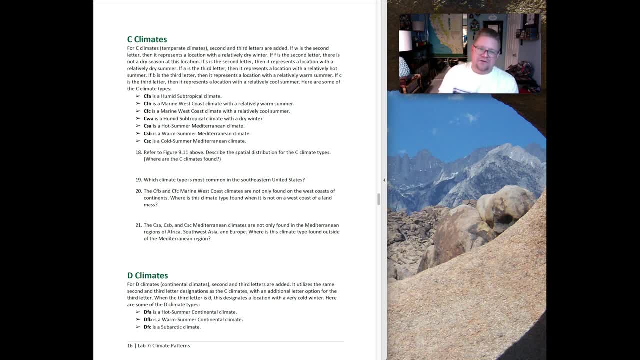 We're comparable to Greece, which is pretty interesting, that we're in California, that we have that. So again, correlate those locations, drag them up to the map and be able to answer those questions about what you feel or think about in those observations and interpretations. 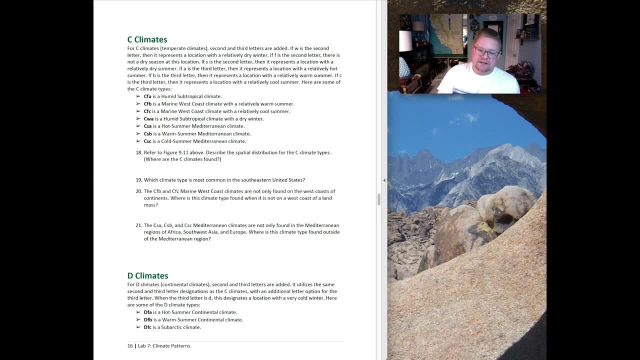 D climates are continental climates. Second and third letters are added. again, It utilizes the same idea, but this time we're looking at places. When I think of D climates, I think of places that genuinely get seasons In most of California if we go from one season to the next. 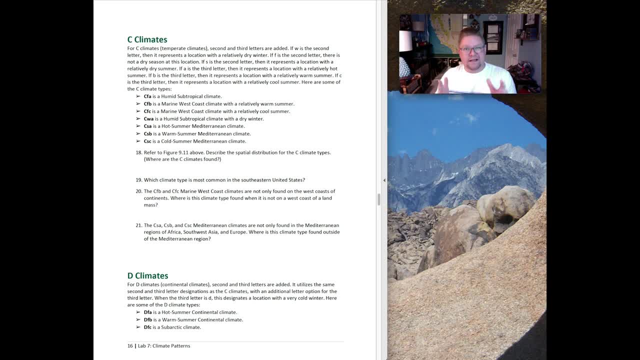 it's like two days It's over Other places. they have like weeks of fall and months of winter and they get all the kinds of these steps, that kind of work their way through. So they go from nice having summers and having very frigid, freezing winters. 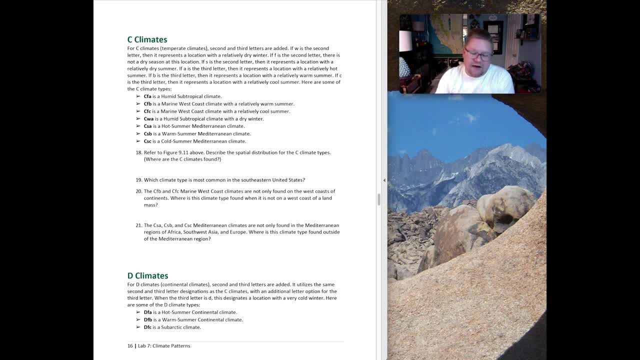 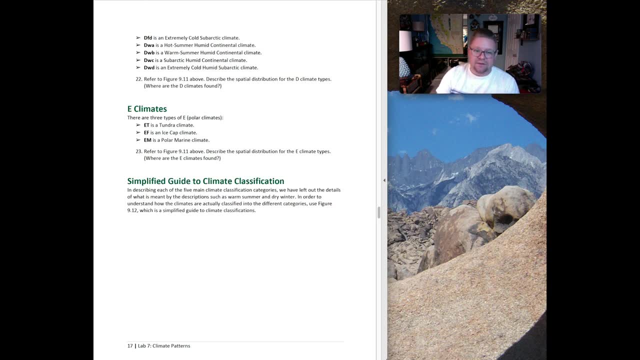 with snow in their front yards and snow plows, things that I've never had to deal with here in California. That's what I kind of think of areas like that. And then last is going to be E, which are polar climates. Some groups also use F for highlands and stuff like that. 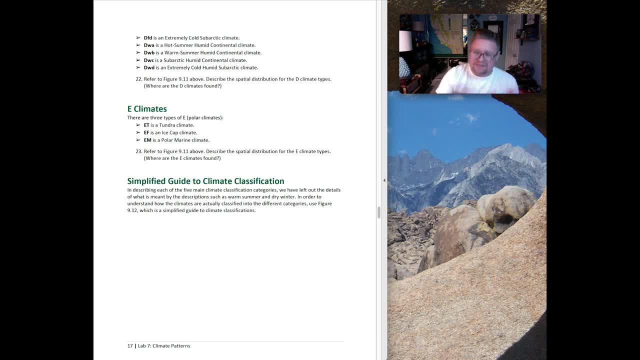 but this group isn't using it, So we're really simplifying. just these main ones, A through E, Again describe what you think. What's interesting again about E climates is that it is polar climates. We know that polar climates can be very similar. 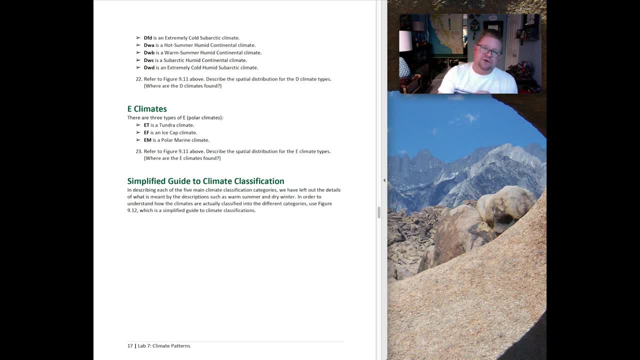 to desert climates because it's as a very minimum amount of precipitation, but this time they're taking temperature into consideration. So a simplified guide to climate classification. Again, this is where I mentioned that build your own adventure. Scott did a fantastic job with this. 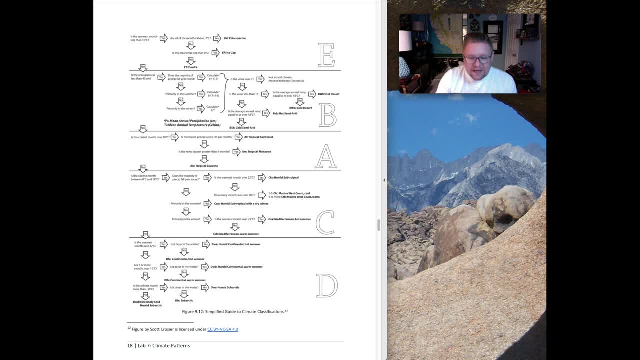 So we're able to kind of work our way through it And by doing so, you kind of work through your patterns. Is this yes, no, yes, no, and you work your way through. So, thinking just simplistically, using your home as an example. 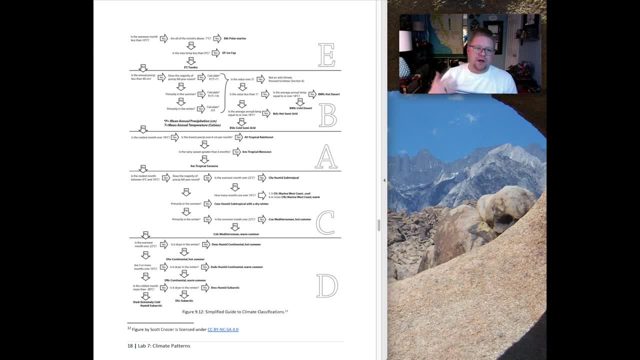 when walking through. this Is your warmest month- less than 10 degrees Celsius. If the answer is yes, you go over here and you get to choose one of these two options. If your answer is no, you drop down to the next letter. 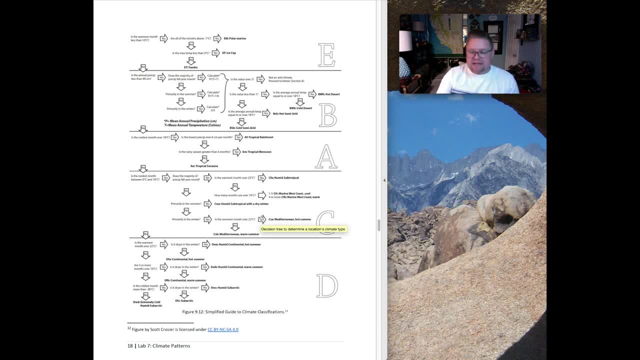 and you keep doing that. So, as an example, like I said, you were in Santa Clarita, I'm at a Mediterranean hot summer, So I would have worked my way through this table and gotten there. The other thing, just like any dichotomous key. 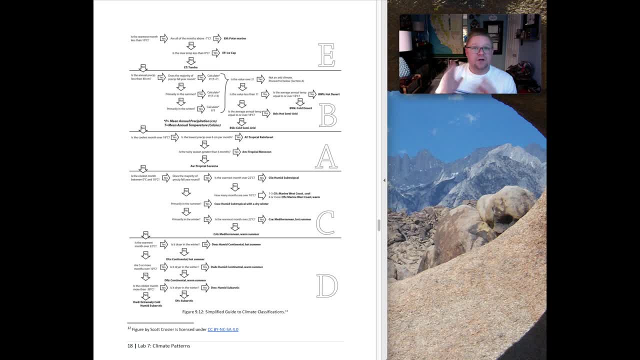 if you find that things are starting to look kind of funky, start over again. It's much easier Now. I was just talking about just applying your personal experiences, But you can actually use something a little bit more specific. What could that be? 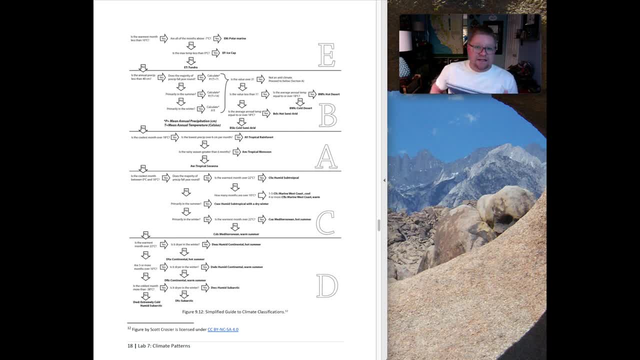 Your climagraph. Your climagraph provides generalized data, long-term study data and averages, So you're able to see that You're also able to look at your climagraph and go on average. The warmest month is June and it's going to be at whatever degree Celsius. 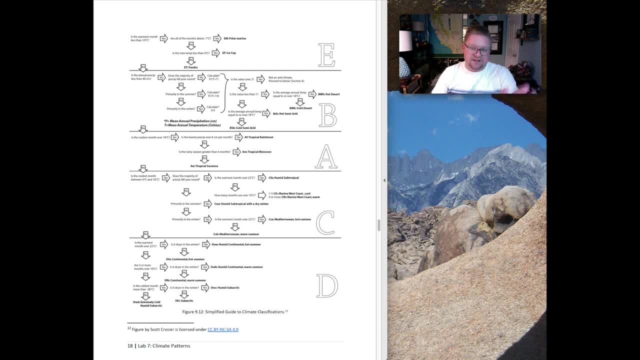 and so on and so forth, So you're able to use a climagraph and this table to categorize a code. Why is that important? Well, it's so important when you're doing research articles and stuff like that, because imagine that someone says: 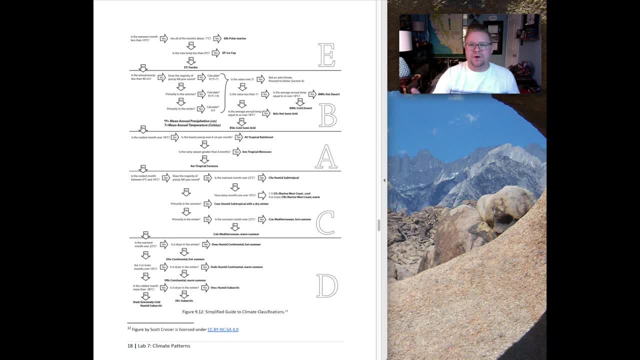 hey, I'm a pen pal from Europe. I'm going to come stay with you for a month. Great, That's exciting. First time to America, This is great. What should I pack for? You could literally give them a two or three code. 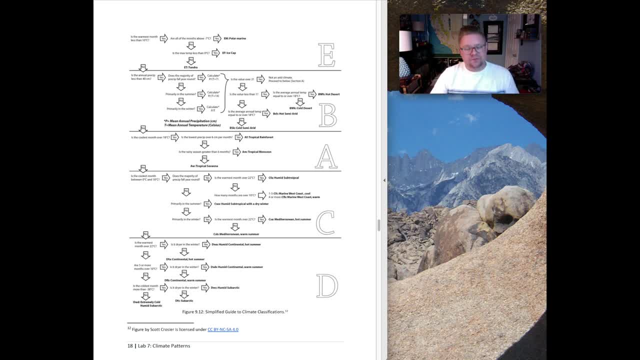 letter code and they would know exactly what your climate is. We don't do that. of course, We like to drag things out, talk about the complications of climate change, The complications of stuff, But that would be the easiest way to do it. 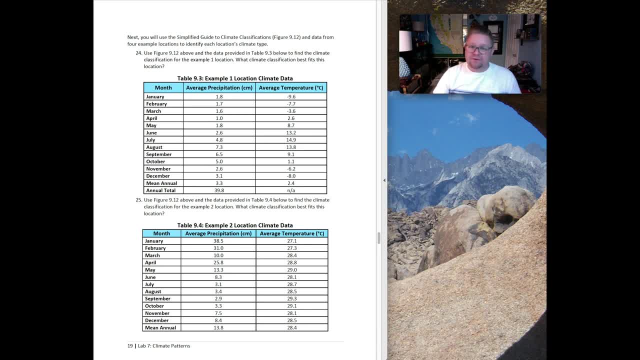 So, moving forward, next you're going to use a simplified guide to climate classification, that table before and the data below in order to essentially give it a category lettering. So it says: use figure 9.12 above and the data below. 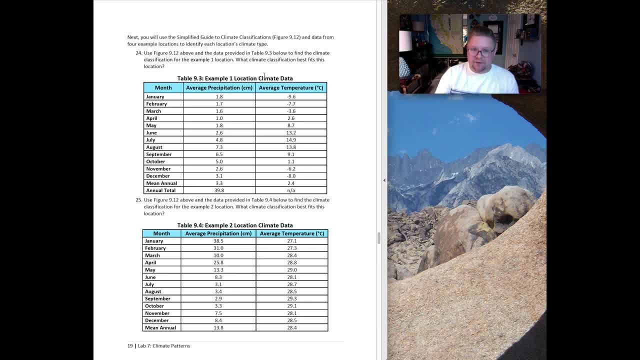 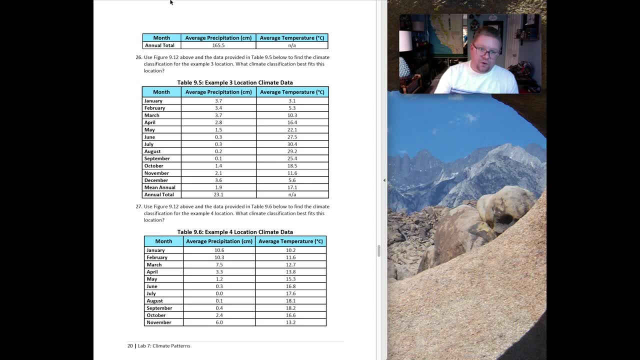 and find out what the climate classification is, for example, location one. You'll do the same thing for location two, Location three, Location four, And then that'll bring us into this next piece, Excuse me. So then we can look at. 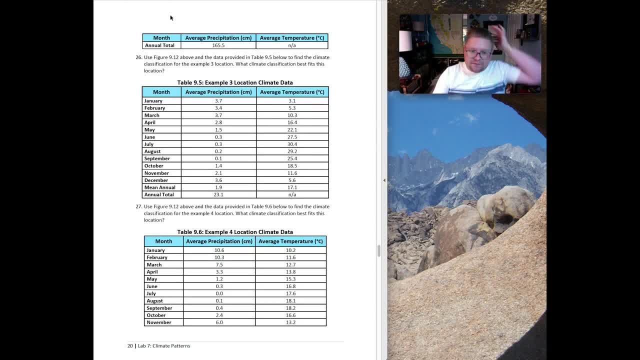 oh, I guess it shifts back up. So then that would wrap you up So you're able to use these datas and data to create your climate classification. Now, I mentioned earlier, California's climate type is really diverse, as we know, You know. 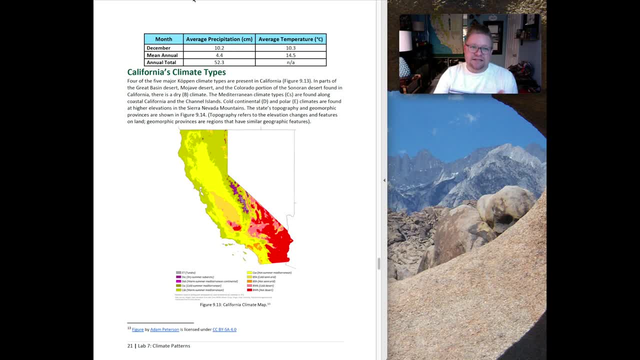 when people say, oh, I'm going to come visit you in California, It's like, oh, what part of California? Because you know, California's climate type is really diverse, as we know. You know, when people say, 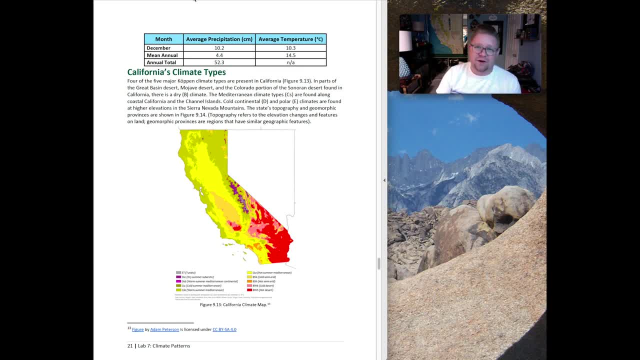 oh, I'm going to come visit you in California. It's like, oh, what part of California? Because you know you could technically go surfing and snowboarding in the same day. So you know, it depends on that region. 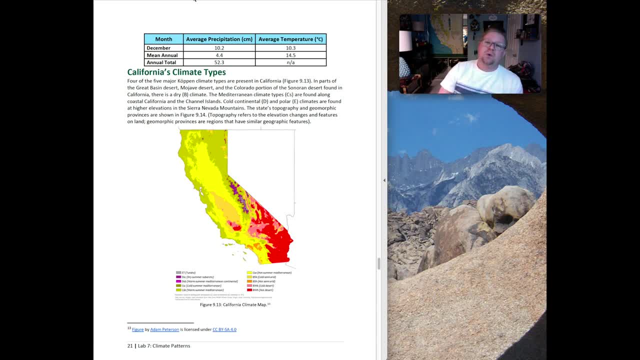 And we find that not only does it have to do with our latitude, but it has to do with our elevation, It has to do with our wind patterns, It has to do with, you know again, those five elements, You know. 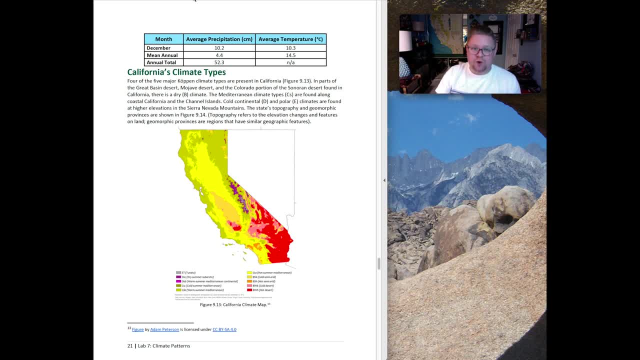 which ones does it mostly rely on in your location? So it says here four of the five major coping climate classifications are present in California, as seen below, In parts of California, parts of the Great Basin, Desert, Mojave, the Colorado. 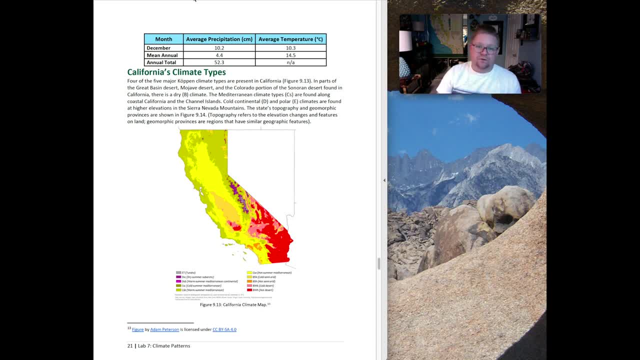 we'll find that there's, you know, tremendous amounts of B or arid climates. We'll find Mediterranean climates, we'll find areas of cold, continental and also climates of higher elevation are also observed, you know, in this map, Like I said, 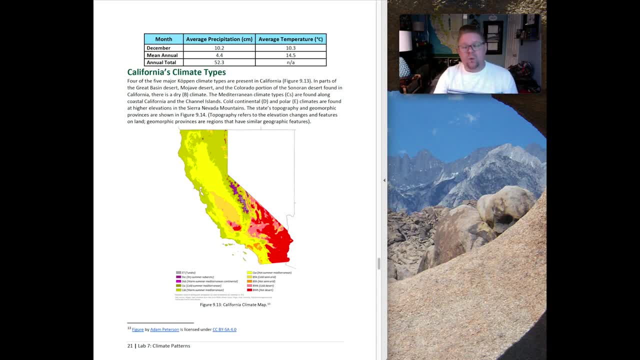 we can go surfing and snowboarding in the same day. So why is this so important for us? Why is California so unique and diverse? We have four of the five major coping climate classifications here. It's because of our, I think. I genuinely believe. 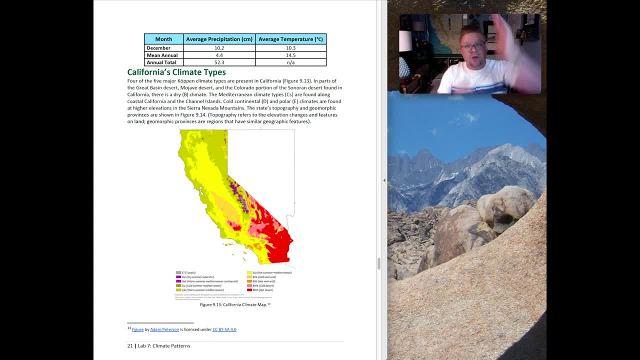 it's because of our latitude and topography and the fact that we are long. Most states are wide. We're long, You know. we transcend all that, So we get to see these different categories in place. So now we're able to observe. 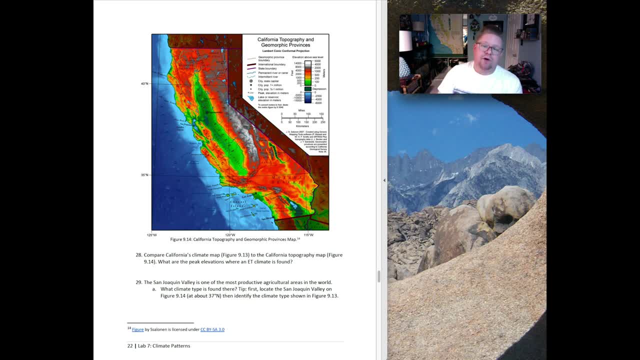 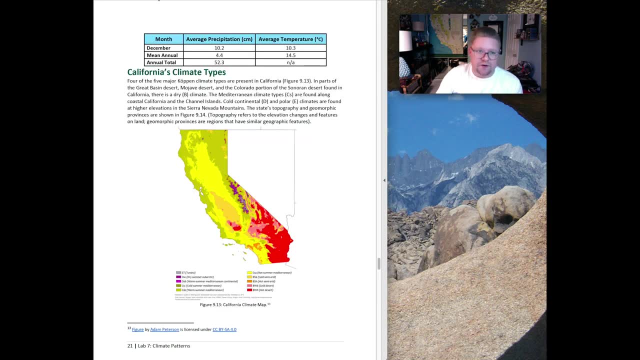 a map of California showing its topography and geomorphic provinces. So we're going to answer some questions that compare both this diagram to and, as well, with this diagram. Do we see any patterns, any observations? So, as an example, question 28 says: 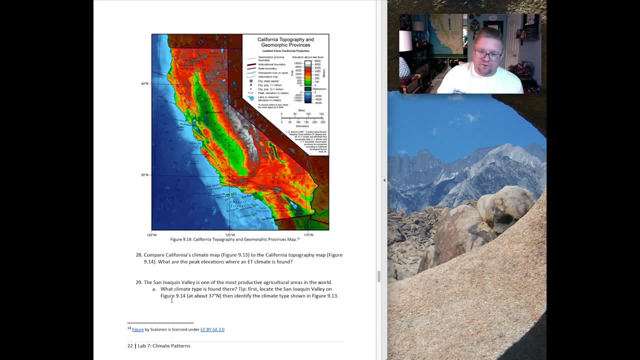 compare California's climate map to the California topography or topographic map that shows the elevations, What are the peak elevations where an ET climate would be found. So you're going to be able to then pull some of those attributes back and forth between these diagrams. 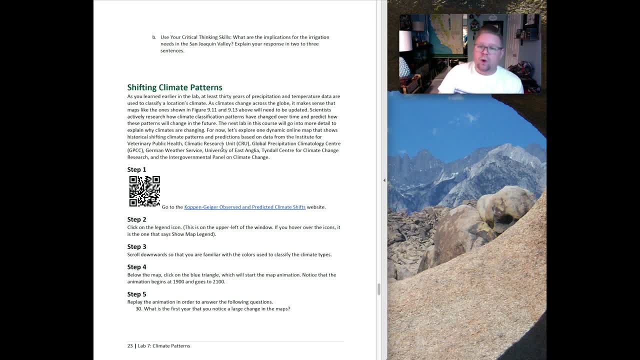 Question B: using your critical thinking skills, what are the implications for the irrigation needs of the San Joaquin Valley? So talk a little bit about that Again, using both the map: the map, the topography map that shows the geomorphic provinces. 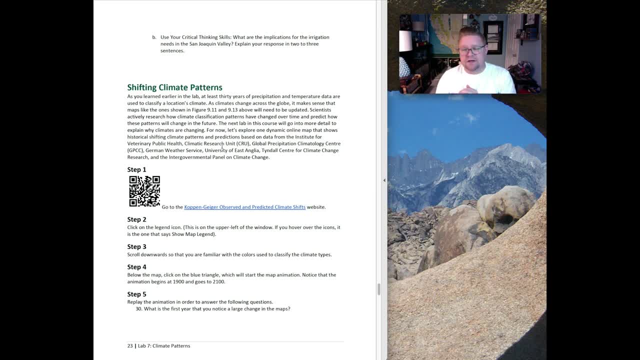 compared to the general climate map, Because we know that the San Joaquin Valley is one of the major contributors for agriculture, for not just the state but for the United States. So what type of challenge do they have? They have all this agriculture. 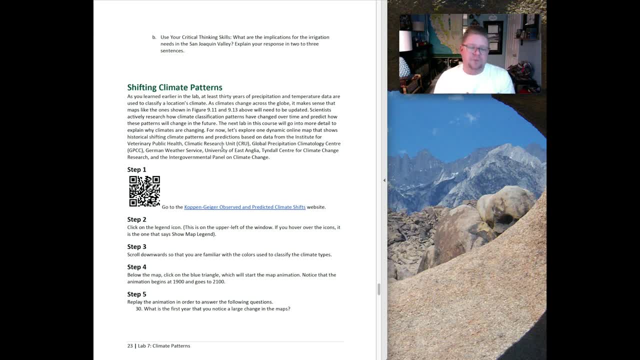 because their soil is so rich, but do they have all the access to the water? And those are some of the observations and interpretations you're going to make Now. shifting climate patterns is a big thing, right, As you've learned early in the lab. 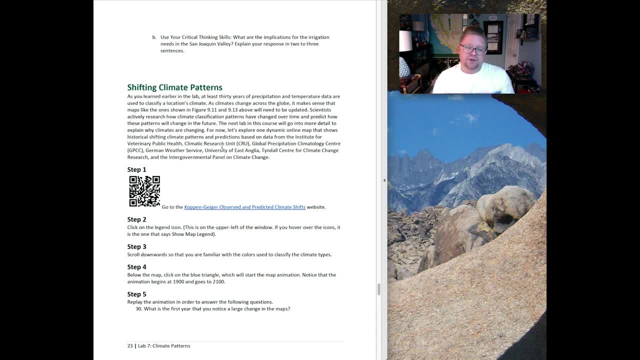 at least 30 years of precipitation and temperature data are used to classify a location's climate. As climate changes across the globe, it makes sense that the maps like the ones shown in figure 3.11 and 3.13 above will need to be updated. 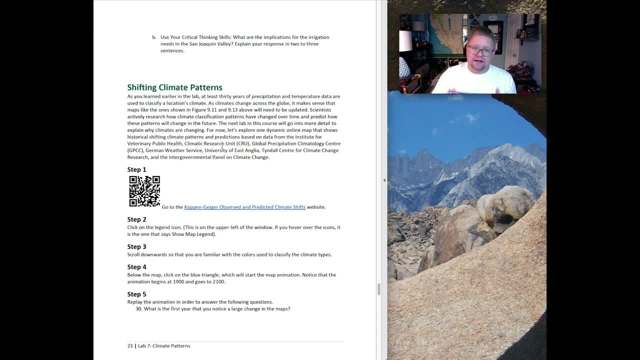 Scientists actively research how climate classification patterns have changed over time and predict, based on those general trends, what it will be like in the future. So what we're going to do is a little bit of an activity. So it says here: step one: 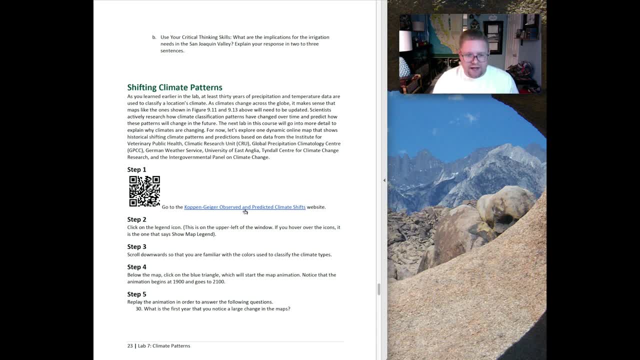 you're going to look at the Copenhagen Observation and Predicted Climate Shift website. So you're either going to take a picture of that QR code or click the hyperlink, and you're going to follow these steps. Step two: click on the legend icon. 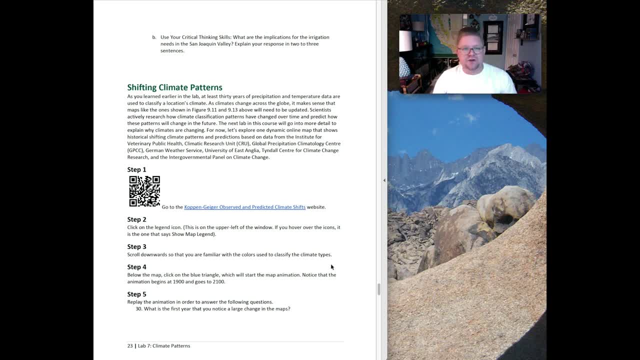 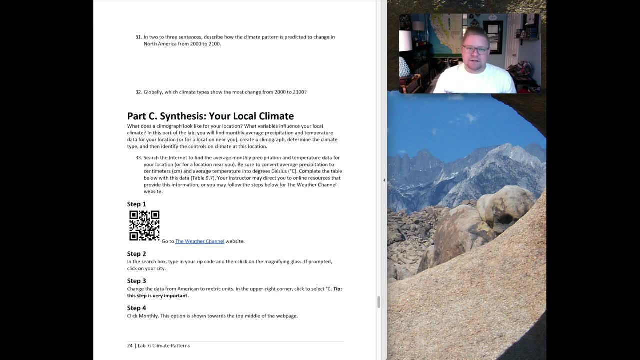 Step three, scroll downwards so that you're familiar with the different colors and how to use this activity. So as you kind of work through that, you'll get a couple questions. 31 says, in two or three sentences, describe how the climate pattern. 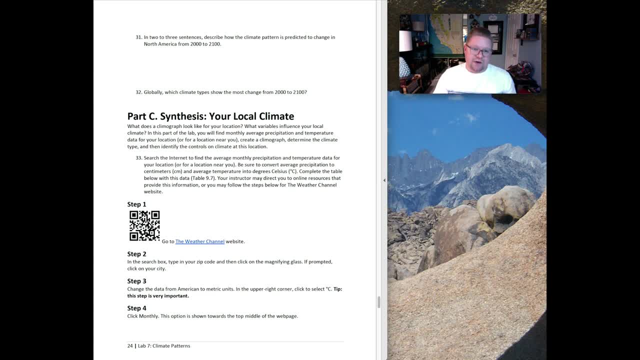 is predicted to change in North America between the year 2000 and 2100.. And then question 32, globally, which climate pattern seems to be the most changed from 2000 to 2100?? And that being said, we wrap up part B. 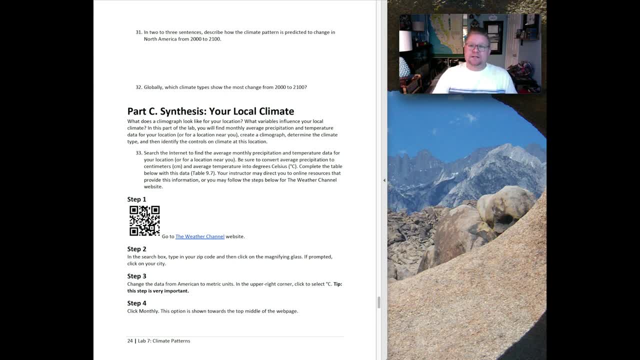 So part C is the final part of this lab. It's the synthesis, your local climate. So what does a climate graph look like in your location? So what you're going to do is you're going to be creating your own climate graph. 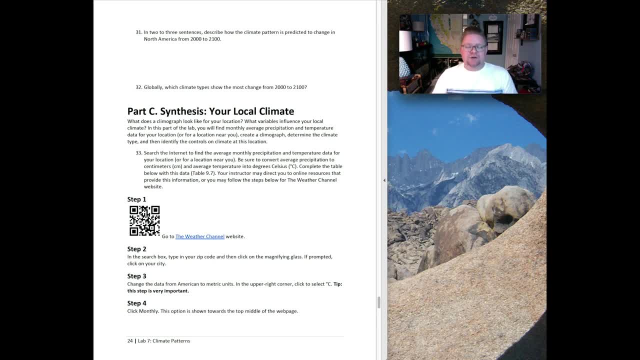 But in order to do that we have to collect data. So the lab itself identifies for you to do: your town, your city, You know. obviously it depends on what your instructor has assigned, if they've picked someone somewhere in particular, But for the most part, 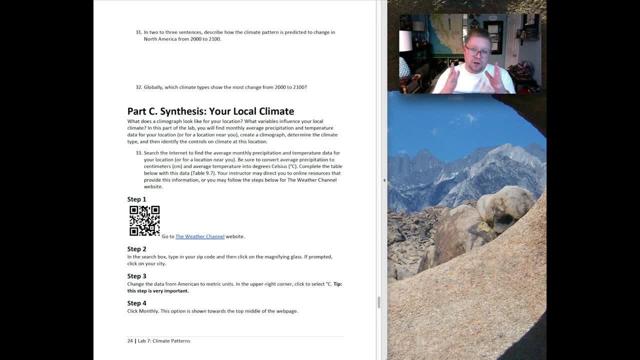 we're looking at just. can you create a climate graph for your location or your home? So the first part says question 33, search the internet to find the average monthly precipitation and temperature data for your location. Once you do so, be sure to plug it. 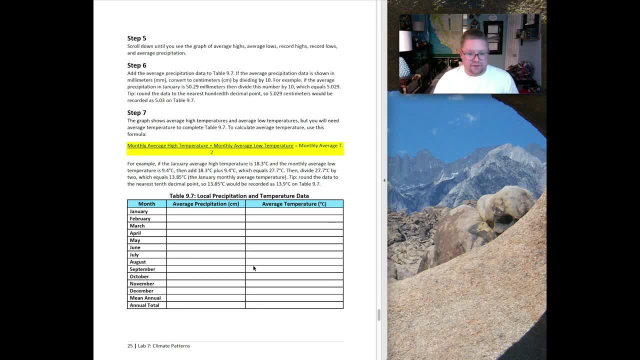 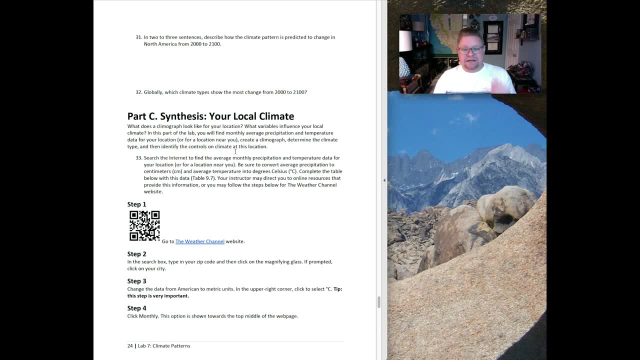 into the table on the next page down here. Now, the key to success is that chances are it's going to be in Fahrenheit and also going to be in inches. You need to convert it into Celsius and into centimeters, So make sure you do. 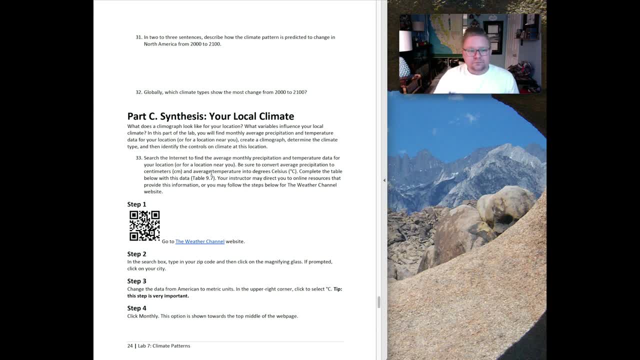 that on that table. So then it says your instructor may direct you to an online resource that will provide this information, or you may follow the steps below. So what ends up happening is, if you can find it elsewhere, or your instructor tells you to find. 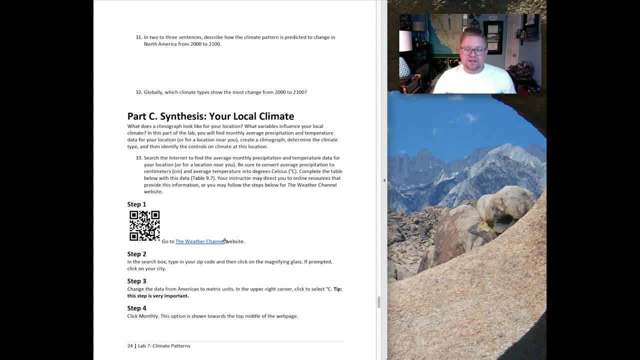 it elsewhere, great. If it's not available, then this is where you can actually access it. You can get it from the Weather Channel directly, So it teaches you to do that. The only caveat would be is that it's not going to. 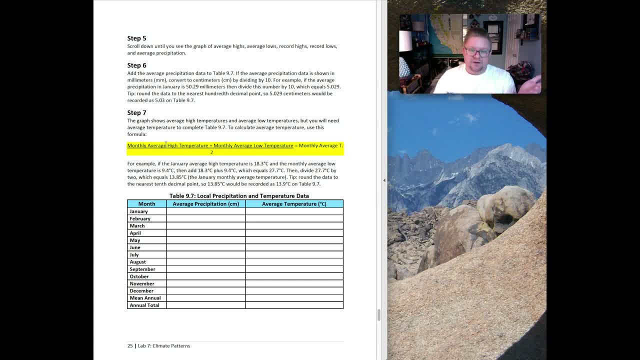 give you averages. You'll have to solve the average, which is super easy. The average is going to be the high plus the low and divide it by two. But some places have data readily available. Some places don't. The other thing to take in consideration. 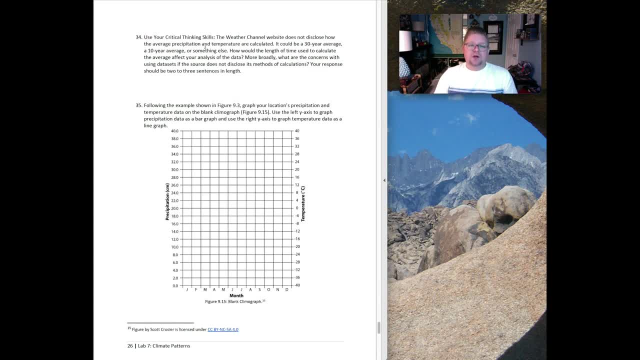 which I believe is actually on the next page. Let me see, Yep, That unfortunately the weather data does not always use 30-year data. Sometimes it can be 10 or 20 or something else. It depends on how long they've been. 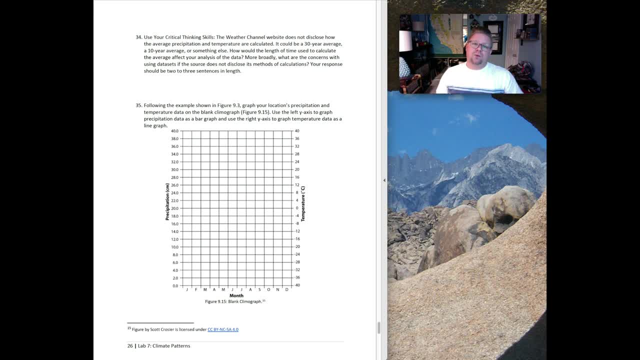 collecting data, if there's been a weather station there that long. So it's asking you what challenges or what fallacies or what problems might you come with if you know, maybe your data is only a two-year data. Is that going to? 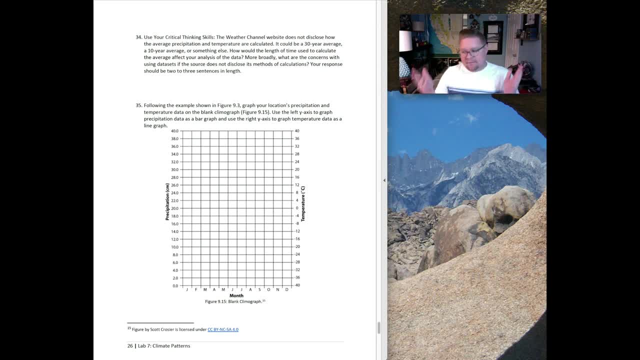 really provide you a generalized amount of information to understand the average climate or to see if there's been change. Question 35 says: following the example shown in Figure 9.3, now you get to graph your own location of precipitation, So you use that data. 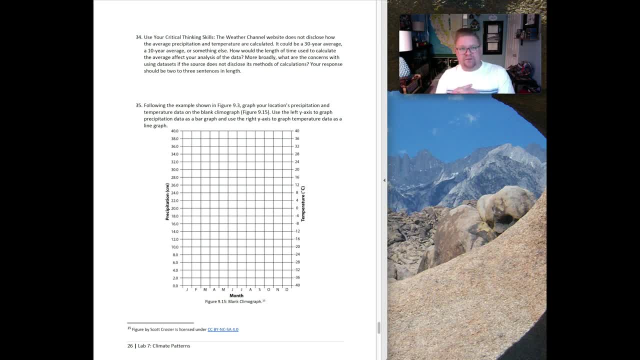 from that table above and you're going to plot in a bar graph- you know the bars- your precipitation values, And then you're going to be utilizing your line to draw your temperature values that are on average for each month And the directions. 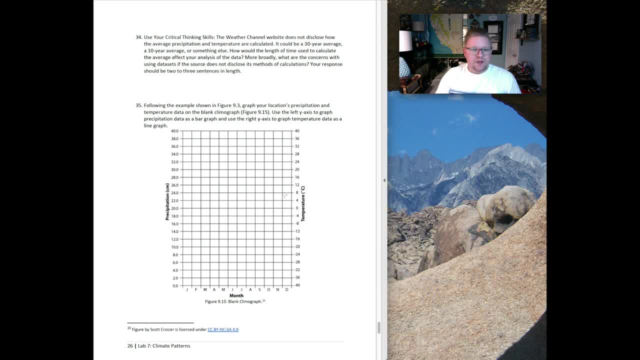 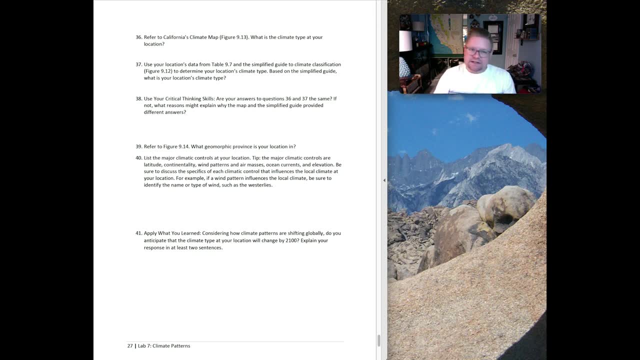 are certainly there to follow through Now. after you do that now, we've got a little bit of information for you. So if you do that now, we've got some references. So you know. question 36, refer to California's. 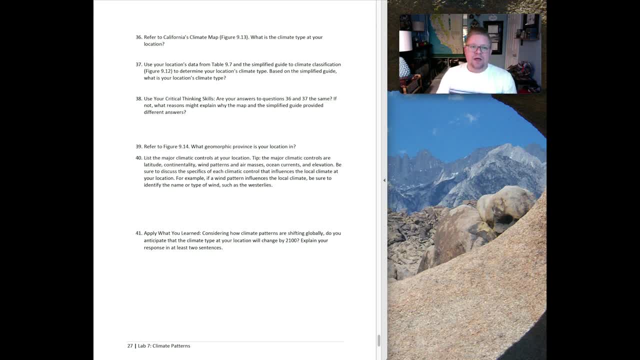 climate map, Figure 9.13.. What is the climate in your location based on that map? Now, using your location's data from Table 9.7 and the simplified guide to climate classification- now you're going to solve your own and see if it's the same. 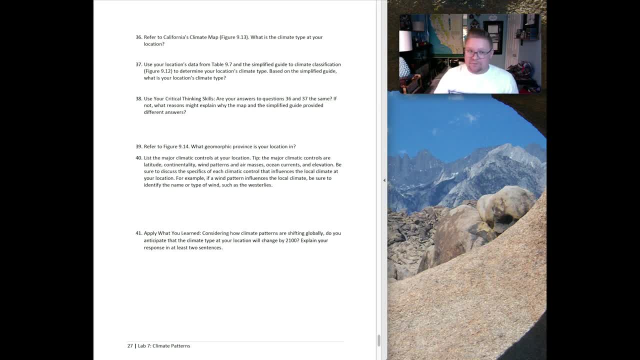 You know, are the answers the same? Are they different? Why do you think it might be different? Why might they be the same? What is the location in? And then, question 40, list the major climate controls in your area. 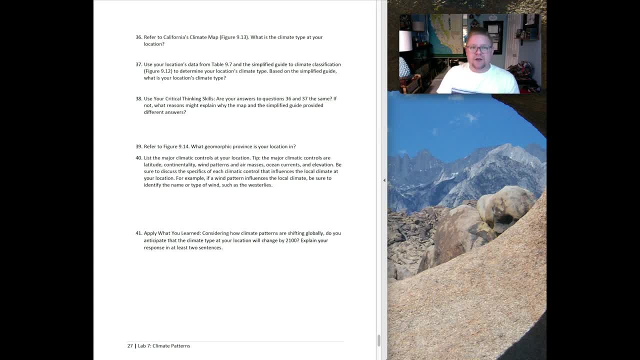 And then it gives you some helpful tips in order to do that. And then question 41 says: now let's apply what we've learned. Considering how climate patterns are shifting globally, do you anticipate that the climate pattern at your location will change by 20,? 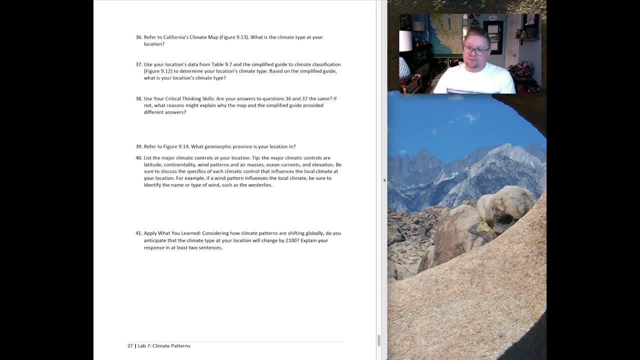 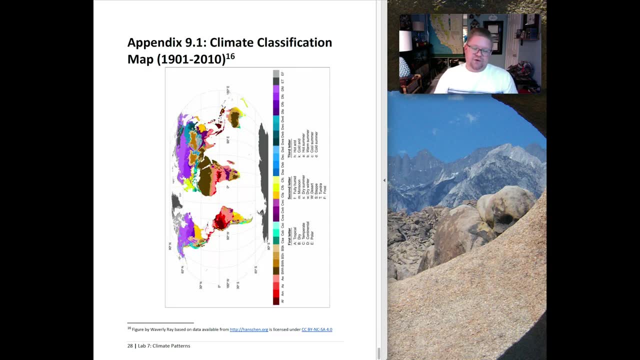 or 2,100? Explain why, or why not, in a couple sentences. Which brings us to the final, last page, which is a bigger version of the climate classification map between 1901 and 2010.. So that's part of your appendix of. 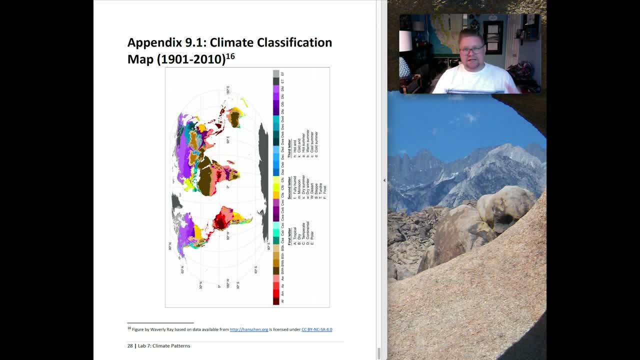 this lab. So, again, this was really set aside to teach you the steps in how to understand climate. When we talk about climate, we're not talking about day-to-day weather. We're talking about day-to-day weather and reflection of the climate. 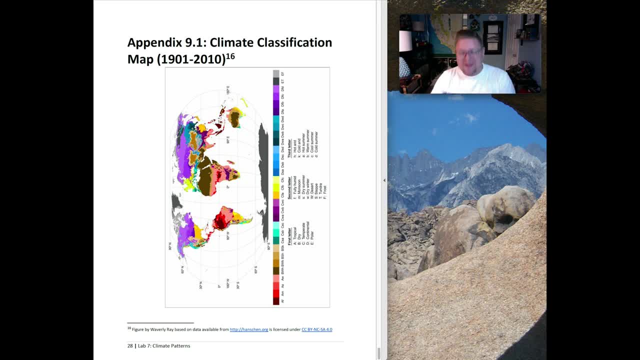 We're talking about the climate classification system and how to research data on your own and to create your own climate graph and then to plot it and solve your own climate classification system for your region. I hope this video was helpful. Be sure if you.